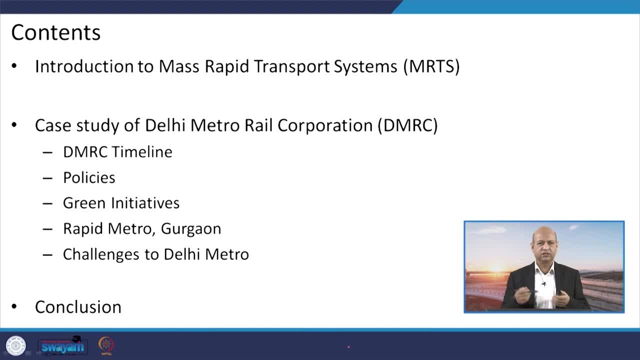 policies, which has affected or influenced the growth of Delhi Metro, And then very good initiatives- or you can say that green initiatives- which has made this Delhi Metro as a wonderful case study all over the world. and then the integration with the rapid metro of Gurgaon, which is a small town now a big town. earlier it was. 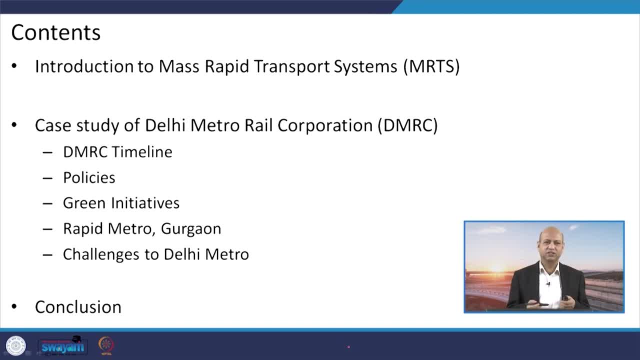 a very small town, but now lot of MNCs offices are there. So it is in NCR, that is, National Capital Region, And this is the town of Faryana. Okay, Okay, Faryana, but just at the border of Delhi. So the rapid metro of Gurgaon, how it was. 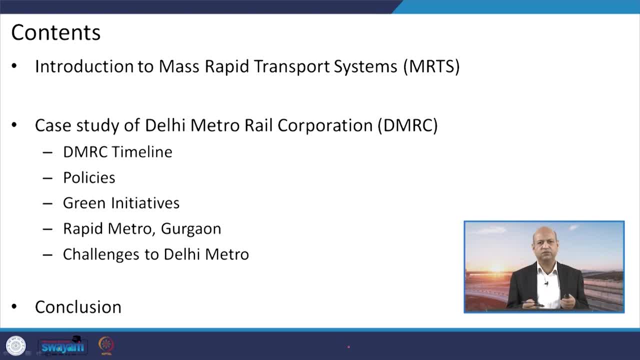 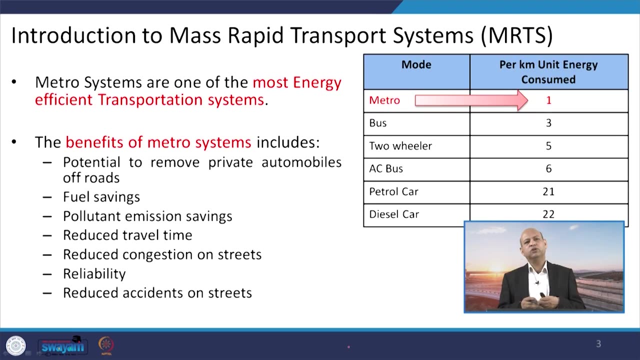 integrated with Delhi Metro. and then some challenges means not all things are very goody goody, but there are certain limitations or challenges or lessons to learn. So those things will be there and ultimately we will conclude this lecture. So, when we talk about 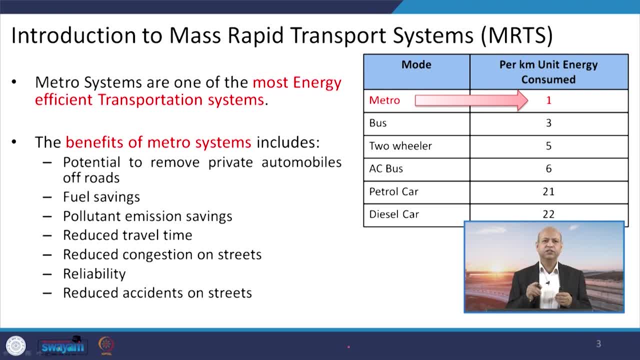 this brief introduction of metro system. you know, basically we will focus upon energy consumption and then the emissions means, exhaust emissions which are avoided by metro system. Now, very small indicator which is very good indicator. you can see, like per. 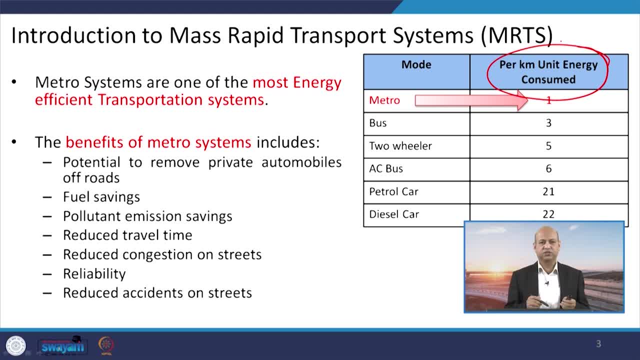 kilometer unit energy consumption. So in moving one kilometer how much energy is consumed by a system like metro consumes? if one unit, then bus consumes three units, see thrice thrice. So dealers five units AC, bus six units, petrol car 21 times and diesel car 22 times. 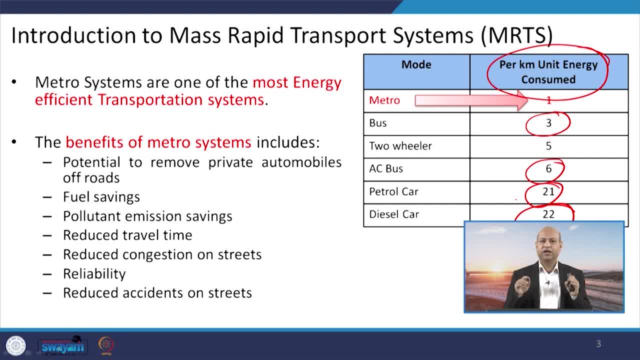 So that means metro is the most energy efficient transportation system in comparison of these other vehicular transportation systems. So there are various benefits in the sense because it removes the need of privately owned vehicles when we shift from that sector to this metro system. 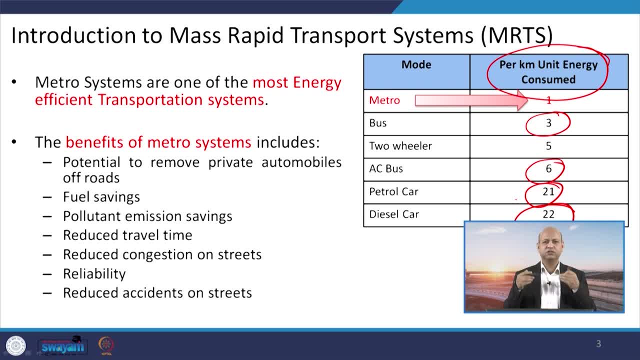 MRTS. and then emission saving, in the sense means those emissions are avoided which were otherwise when we ride the bus or car, Fuel saving is a lot. and then reliability, because the complete system is dedicated corridor. there is no other chances of delaying except. 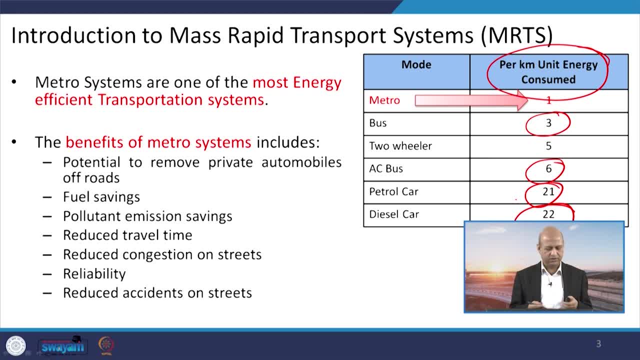 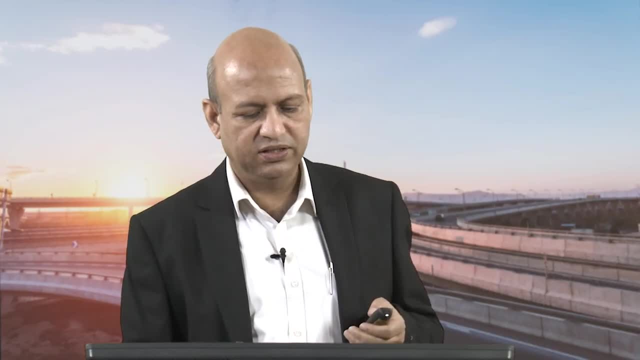 some in a very, very rare case. but that is again means from the reliability aspect. this is one of the wonderful system And accidents which you can see on the roads and streets. there are no chances of such accidents in the metro system. So you can see this one pictorial representation of Delhi. 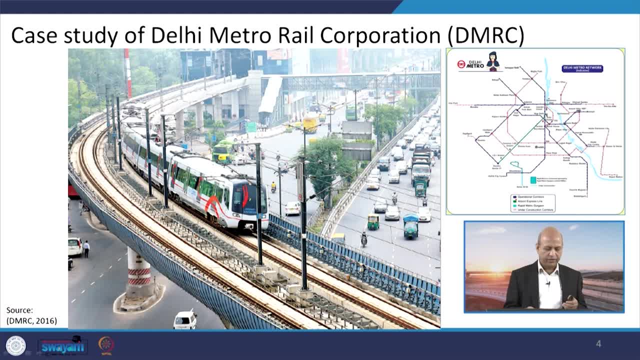 metro, which is the case study for today. So at various places it is elevated and at some places is underground. So this is a mixed kind of in different phases. This Delhi metro was built So in 1995, these controversial works were leading to it changing in price. 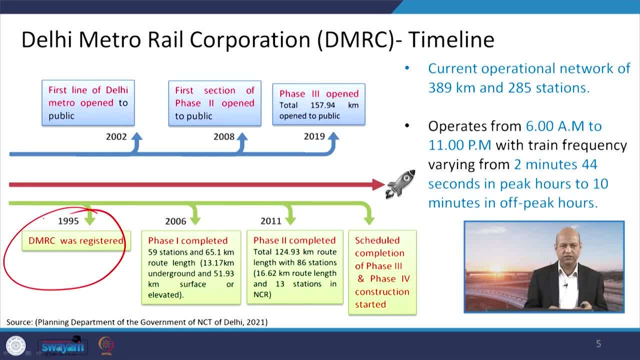 built. So in 1995, this was registered DMRC, that is, Delhi Metro Rail Corporation. the timeline is represented here. In 2002, this first line of Delhi Metro was opened for public. In 2006, the phase 1 was completed and around 59 stations were covered and 65 kilometer. 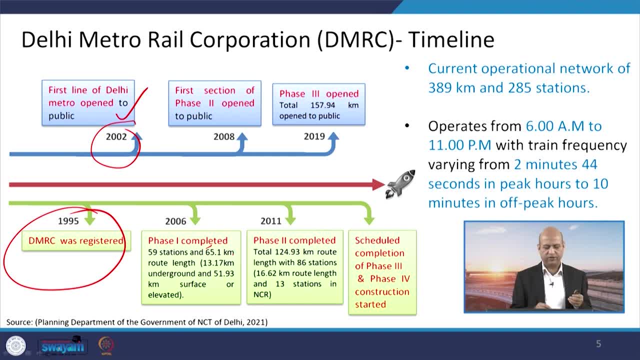 route length was achieved by this phase 1.. In 2008,, first section of phase 2 was opened. In 2011, phase 2 was completed and it could cover around 125 kilometers stretch or the route, and 13 stations were in the NCR means outside Delhi, but in national capital region. 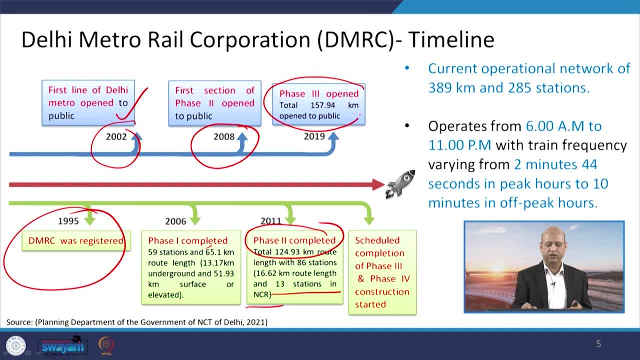 And then in 2019, this phase 3 was opened, total around 158 kilometer and this was open for public. So now this phase 4 is going on and you can see the total network. current operational network is around 389 kilometer, means approximately 400 kilometer with 285 stations, and it runs. 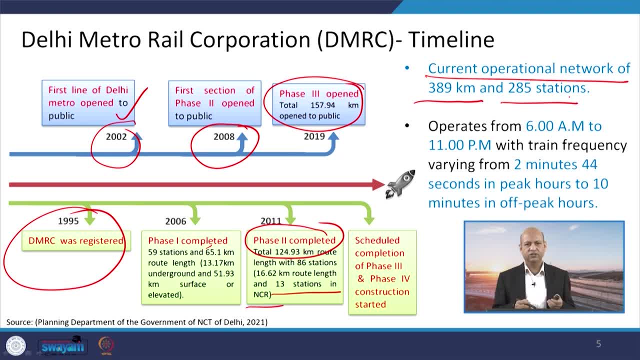 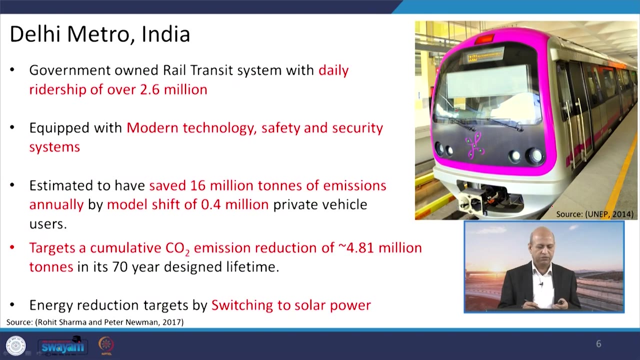 from 6 am in the morning to 11 pm in the night and during peak hours when lot of people are traveling, then the frequency is quite high: every 2 minutes and 44 second one train is there one, and in non-peak hours around 10 minutes is the gap of these metro trains. 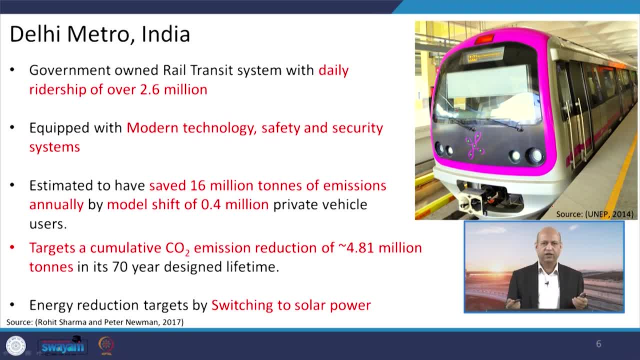 but means that is not a huge gap: you can have your next train if you just miss the first one. Well, the ridership is very large, like 2.6 million people daily Using this Delhi metro, and it is equipped with very high, reliable technology of modern 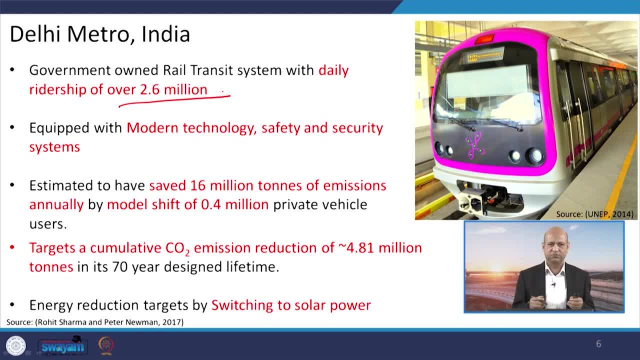 days in terms of safety and security systems. And then if you see in terms of emissions, 60 million tons of emissions annually. it is reducing because of model shift of around 0.4 million private vehicles. so that kind of emissions saving is there. 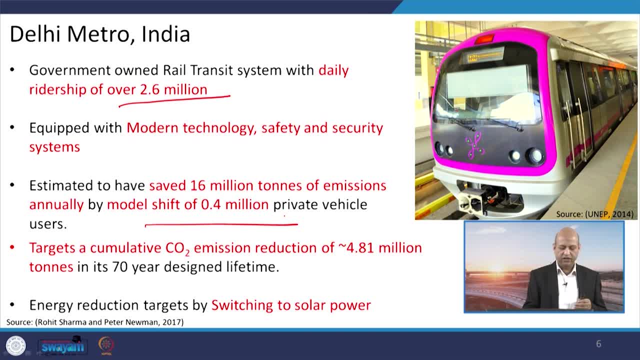 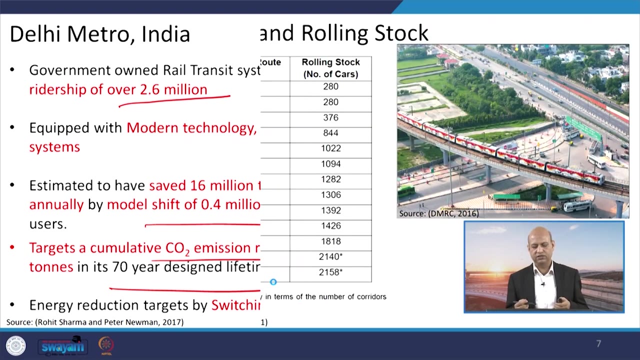 Well, target of cumulative CO2 emissions reduction around 4.81 million tons in its 70-year designed lifetime. So this is estimated figure. and solar power is also being inbuilt or integrated in the whole system so that it can have the renewable resources integration and that way further. 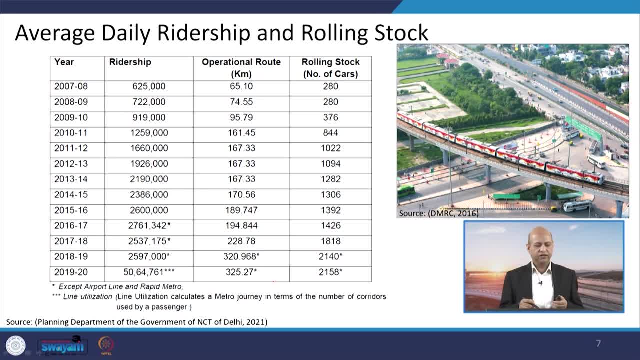 reduction in emissions. Well, you see this. Well, you see the ridership increase from 2007 to 2019, so around 625,000 ridership was initially in 2007,, but now it is 50,, 100,000 or 51,000. you can say operation route. 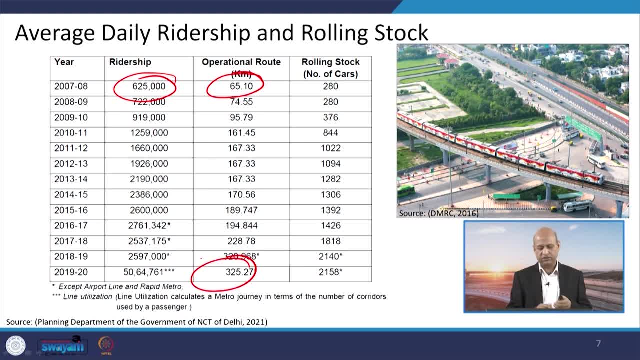 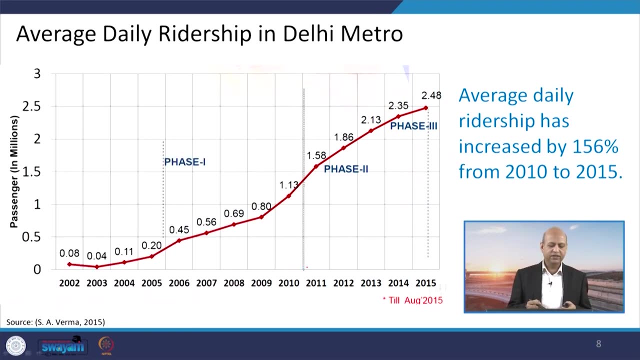 from 65 kilometres to around 325 kilometre stretch is covered. and the coaches or cars: earlier it was 280 and now it is around more than 2100.. So the growth you can visualise with these numbers, plus the ridership, is increasing. 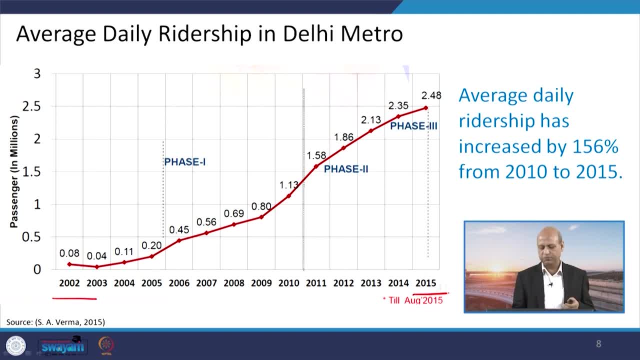 every year from 2002 to 2015,. if you see, the graph is always increasing. That means the people are feeling incentive to ride the metro because of its comfort level, because of its efficiency, because it reduces time to travel from one point to another, and 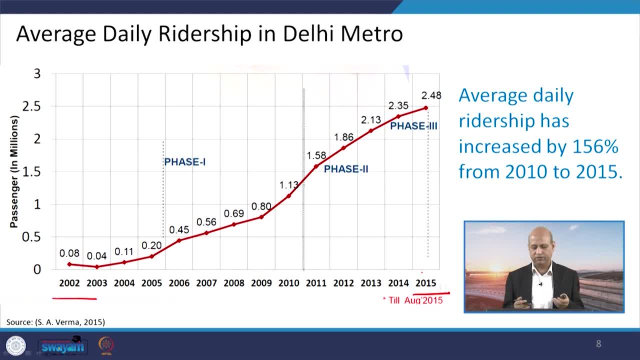 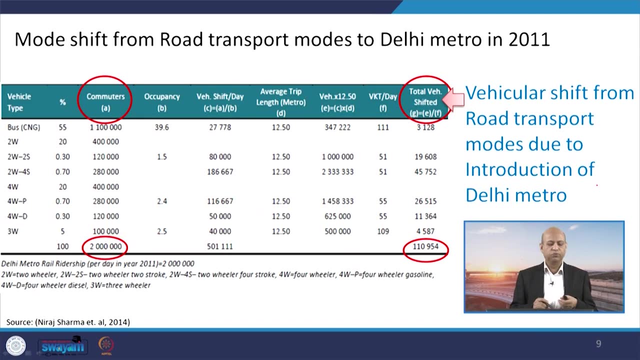 it is completely air conditioned, So that way people like to use it. So it has increased around 156 percent in between 2010 to 2015.. When you see the mode shift from road transport modes to Delhi metro in 2011.. 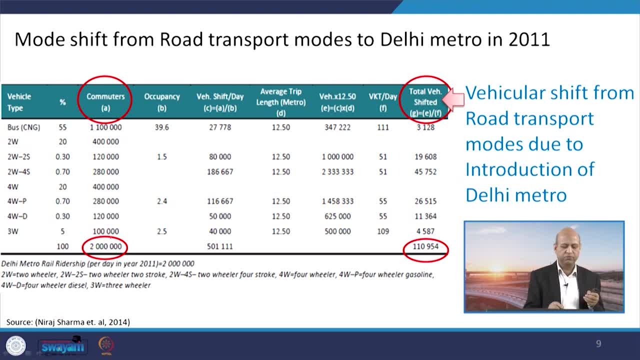 So again you can see the total 2 million. 2 million commuters were shifted towards metro from. like 55 percent people were from buses and then 20 percent from two wheelers, So that way the total 100 percent. the figure was around 2 million. 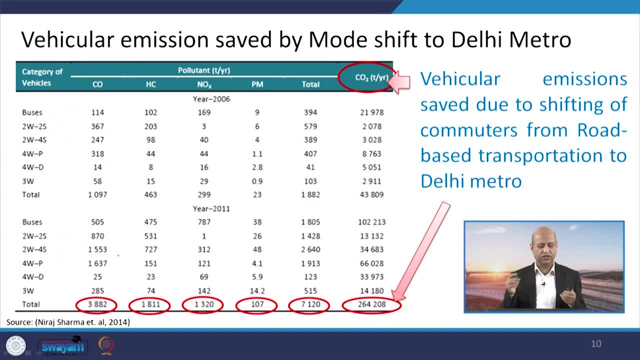 So this is the growth story, but the 2011 figure itself says that it has been very popular, If you see the vehicular emissions saved by mode shift, because when we are going from fossil fuel based road traffic to Delhi metro, Then naturally we are reducing the emissions. 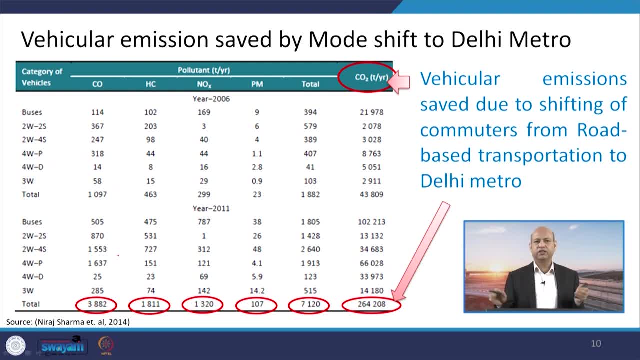 So this is the growth story. So this is the growth story. Delhi metro is reducing the emissions, the exhaust emissions, because Delhi metro is run by electricity, although, as I narrated in one lecture, that people argue that electricity is also produced by fossil fuels, by coal power plants. 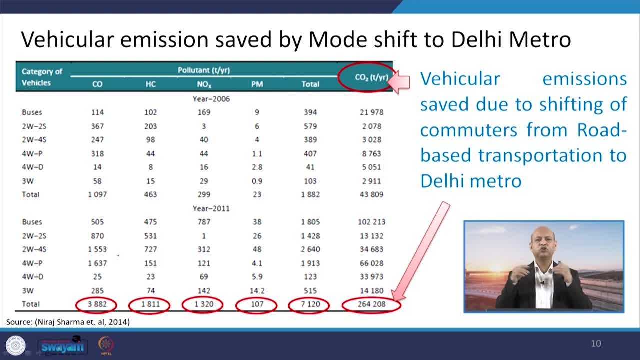 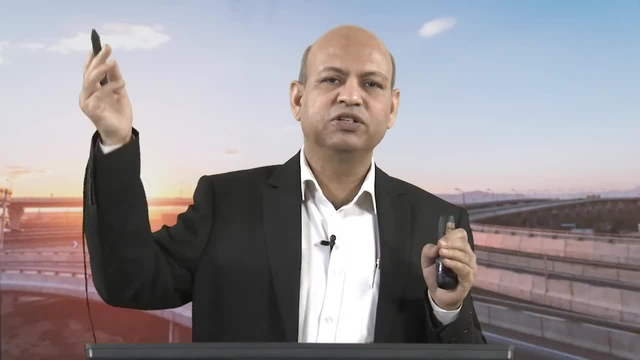 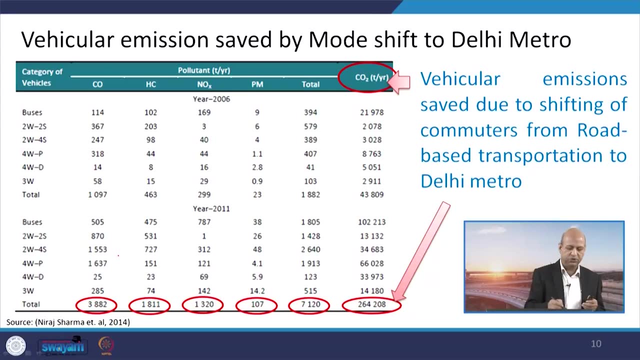 But, as I said, because the vehicular pollution is in the range of our breathing process. So that way the health benefits are much, much more, because the stack emissions get diluted when they reach to the ground level. comparison is not so straight, Anyway, if you see the CO reduction from different categories of vehicles like buses, etc. so 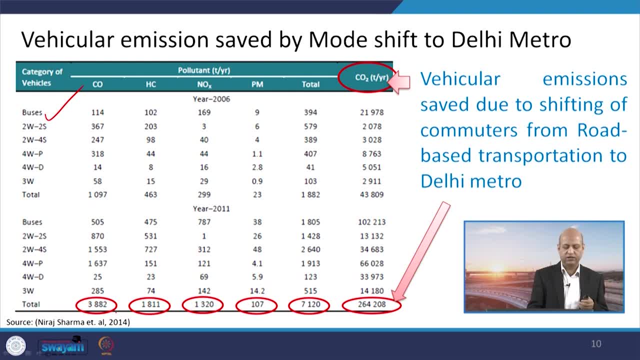 around 3,882 tons per year, saving of CO. similarly, hydrocarbons or NOx emissions, particulate matters, so total is around 7,000 tons per year reduction in the emissions of air pollutants, If you focus on greenhouse gas emissions, or you can say carbon dioxide CO2, ton per year. 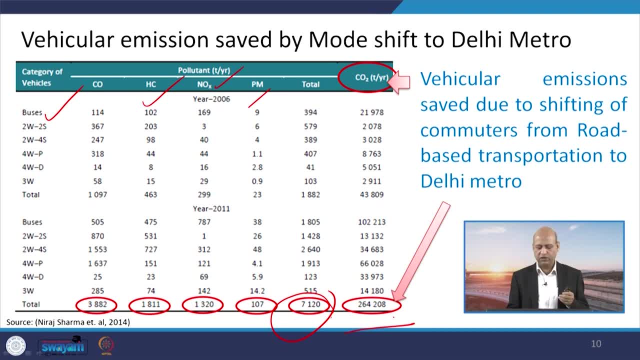 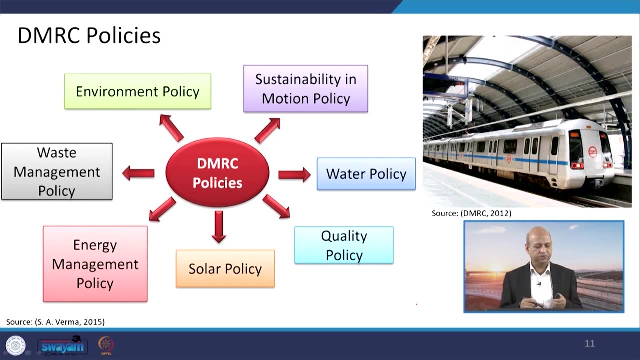 so you see the huge figure of around 265,000 around means it is 264, but it may be around 265,000 estimated figure. it is there, it is not absolute value. So those emissions have been avoided because of this METRO. 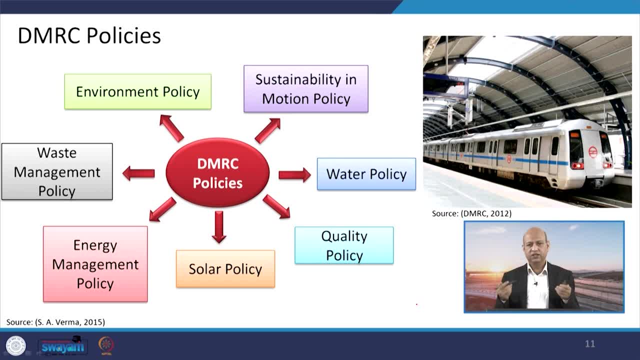 What are the different policies which have been integrated to make it very popular? Because environment policy is there. how to make it environment friendly, we will see different aspect later on. Then sustainability in motion policy means again the reliability and punctuality, all those things. 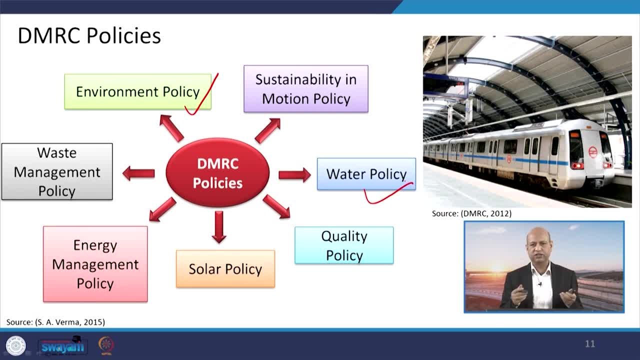 Water policy. we will see that, how recycled water is being used and how it is really using the wastewater treatment through wastewater treatment plants, etc. Quality policy: the quality control is there in terms of Comfort level as well as timings. Solar policy means solar energy is being integrated and energy management policy means several. 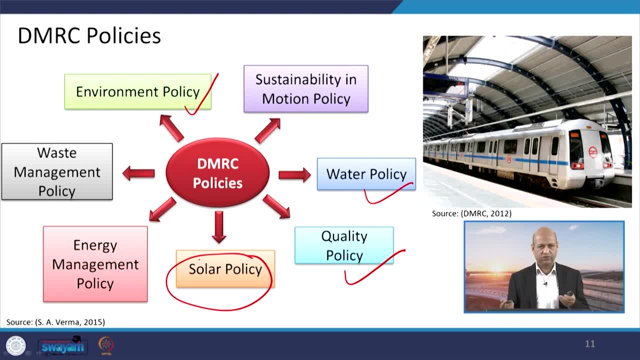 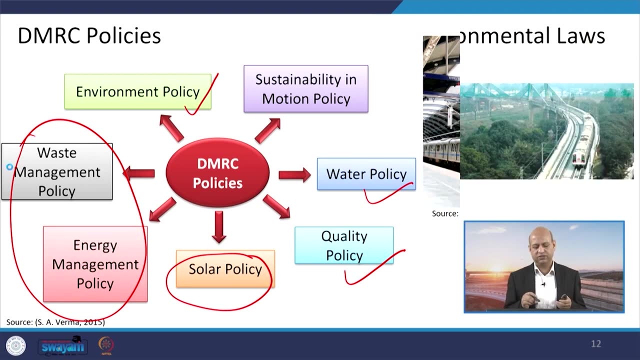 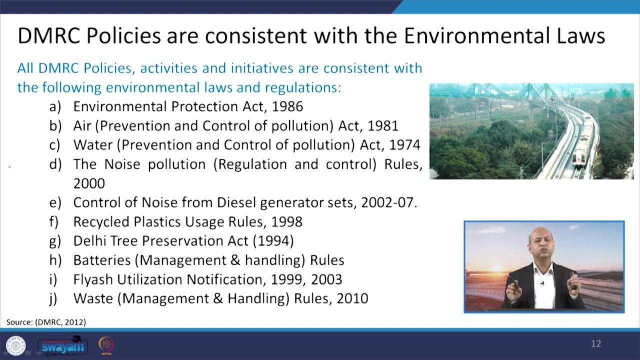 kind of energy sources, even waste- to energy resources are there. So the waste management and energy resources are being integrated. so that way this DMRC policies is wonderfully linked to each other to make it a sustainable case study for transportation systems. Similarly, this DMRC policies in terms of the environment. it follows all the rules. 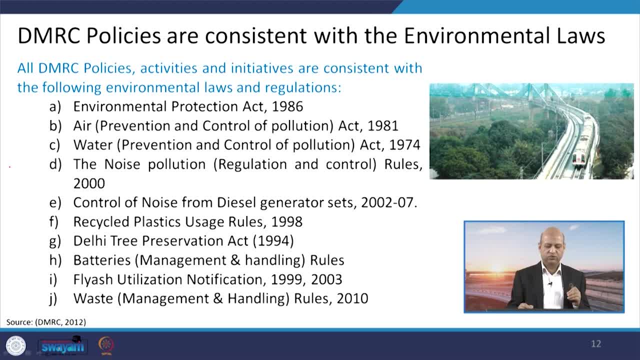 and regulations or environmental laws of the land. So, whether it is Environmental Protection Act of 1986 or Air Pollution Act of 1981, so all these environment related acts and regulations have been properly integrated and implemented in the management system of DMRC. 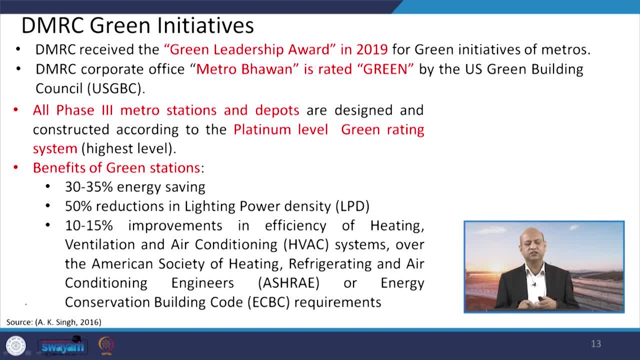 Well, if you see this Green Leadership Award, So the Green Leadership Award of 2009, which was given to Metro Delhi Metro because of its various initiatives for green environment and saving energy, Then this Metro Bhavan was rated, this big office complex, as green by the US Green Building. 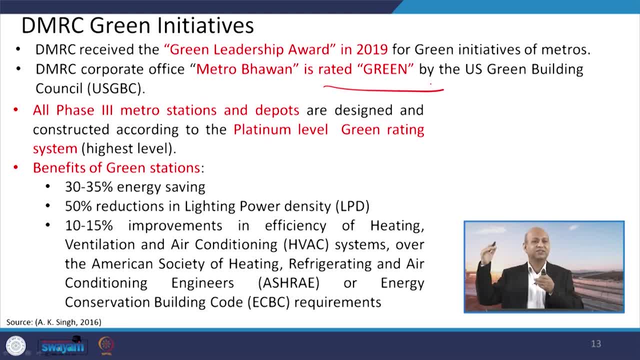 Council. So that way means you can see its standard and practices. best practices of the world have been implemented in the management of DMRC. And then you can see this platinum level green rating system for all construction activities of metro station depots have been integrated and 30 to 35 percent energy savings in all. 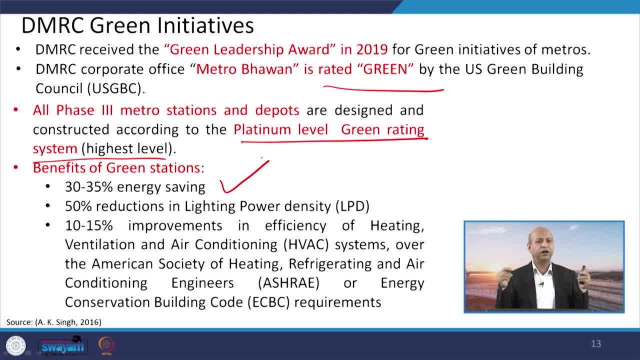 green stations which have been built. So this have been part of planning and execution. 50 percent reduction in lighting power density: all these benefits means whether it is lighting or energy or air conditioning. So reach over the projects. So this is the UNC goal. 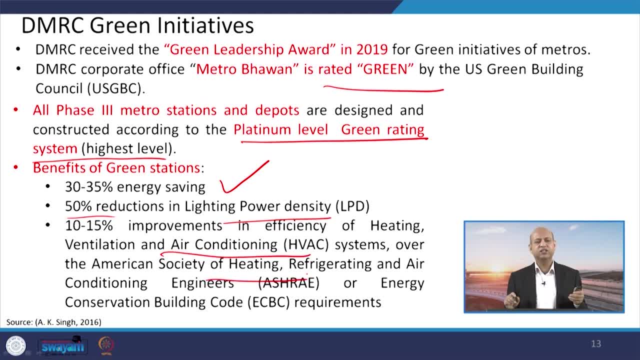 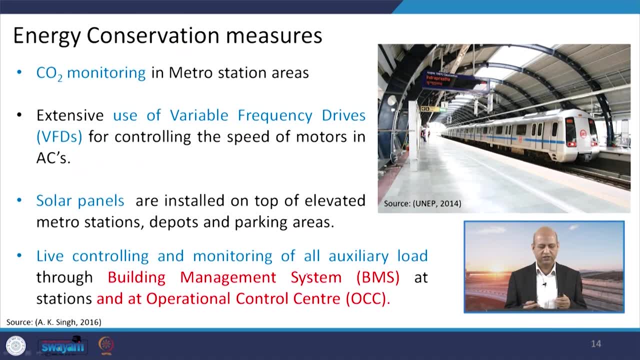 Okay, I submitted thisожалist. this was completed. Thank You very Much. Thanks to BG Somewhere, Pulaam and Sestre system or heating system, all things have been designed as per the best practices of green energy or green rating or green leadership practices. 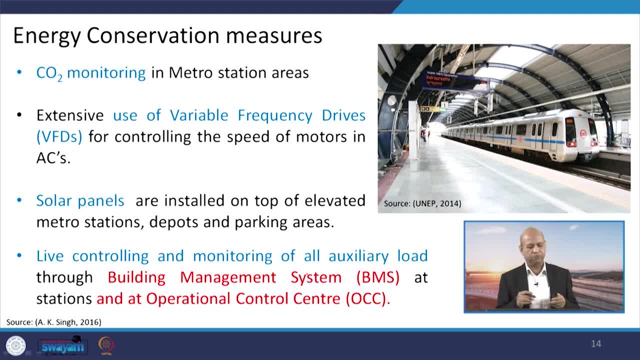 Well, energy conservation measures have been in place, like CO2 monitoring at metro stations, areas. automatic systems are there which measure the CO2 levels so that it should not increase beyond certain level, and there are ways to control it. Then there are air conditioning systems, and solar panels are also there. plus, there is 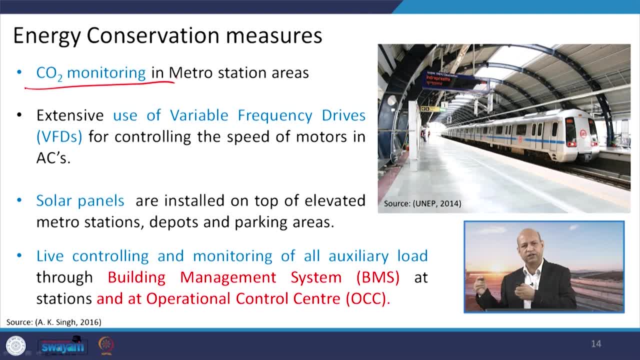 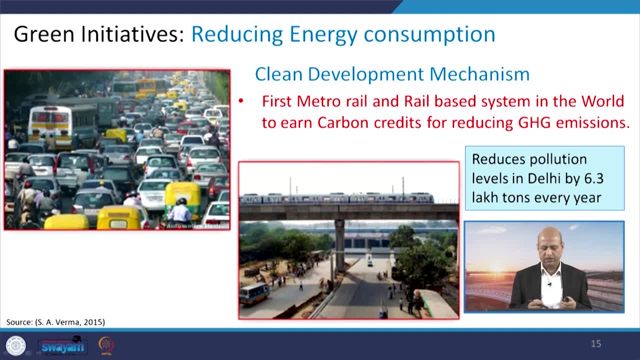 management of air flux between underground tunnels and how this metro goes, and then there is push of the air from behind and it adds to the fresh air. you can see Well this green initiatives. if you compare this kind of scenario earlier, when all these 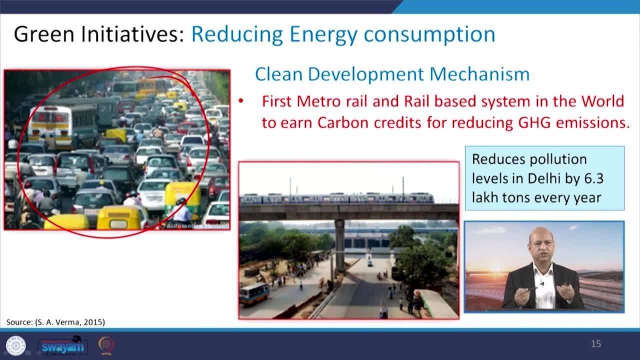 fossil fuels were there. So these fossil fuel based vehicular categories or vehicular, these automobiles etc. are there. they are burning lot of fuels and they are emitting lot of, whether air pollutants or greenhouse gases, but this is quite clean: there is no exhaust emissions. 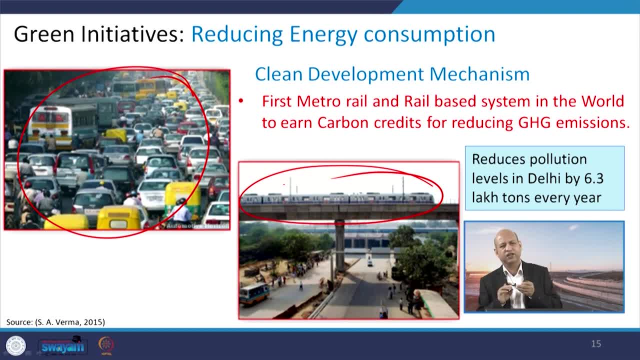 Of course there may be little bit, some like wheel abrasion and friction, very, very minute quantity, but in comparison to this This is kind of negligible. and there is the reduction of pollution. around 6.3 lakh tons per year has been estimated with this clean development. 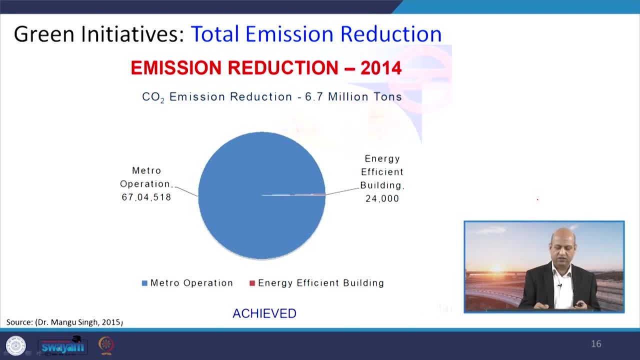 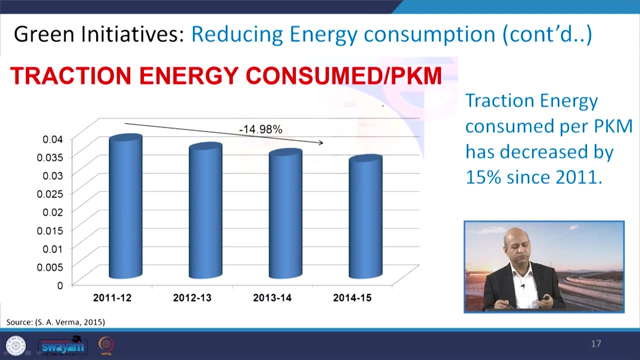 If you see the total scenario, then the CO2 emission reduction has been estimated around 6.7 million tons reduction. that has been achieved in 2014,. this estimated figure is so that is the reduction. Then traction energy consumption, So that is the reduction. 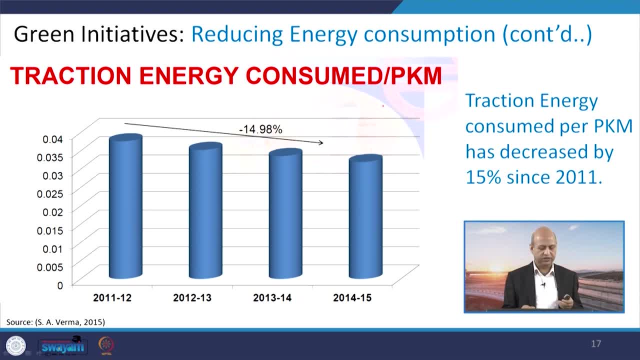 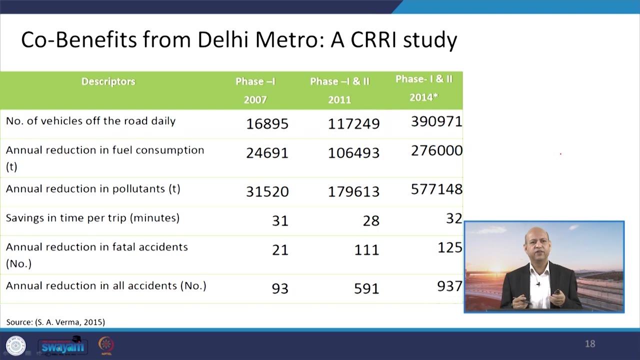 So this is also reducing from 2011 to 2014, if you see so those traction energy consumed has been like 50 percent reduction with respect to 2011.. So those practices have been implemented to achieve these targets. There are several co-benefits also. co-benefits means when some additional benefits become 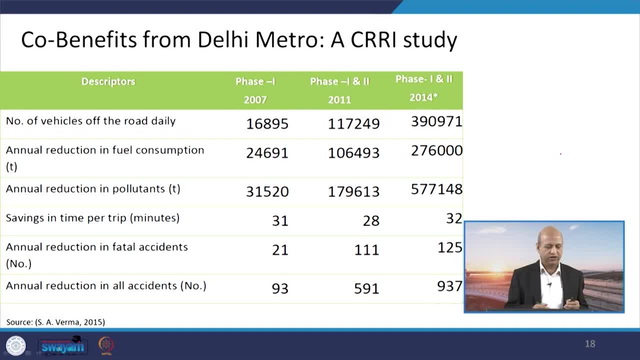 automatically without air pollution, For example, if this annual reduction in fuel consumption- because this is working on electric cars, so in phase 1, this much of reduction is there. phase 2 and phase 4, so it is reduction in fuel consumption is increasing in every phase. 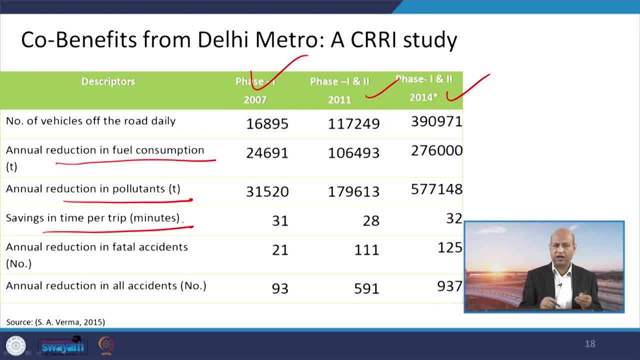 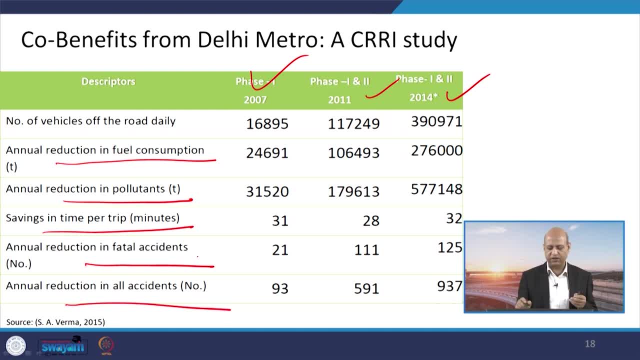 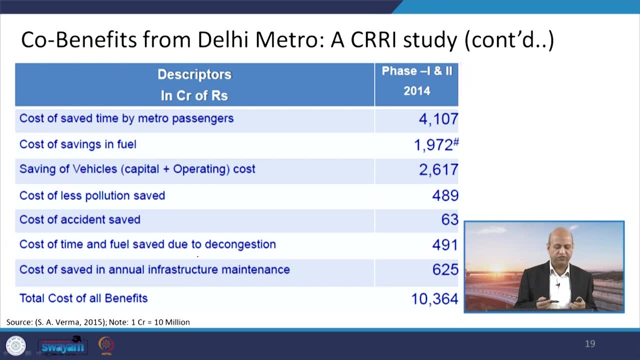 So these are reduction in accidents or reduction in fatal accidents. all those have been increasing from one phase to another one. So this is a success story of co-benefits. Also, if you see the saved time. So that much If you convert it into: 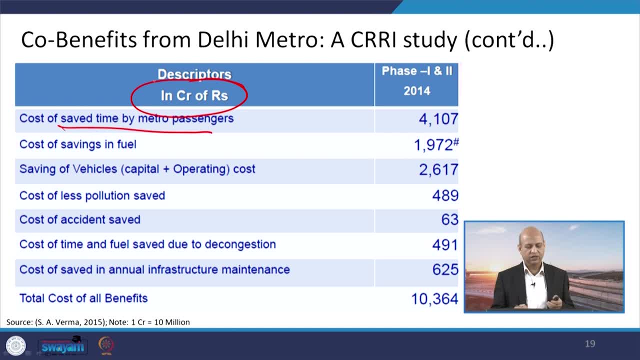 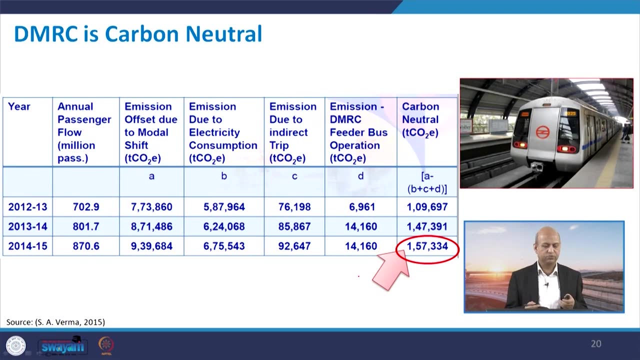 Crores of rupees. 1 crore is 10 million. So if you compare different activities, so the total benefit is around 10 crore or 100 million. So that is a huge benefit if you see in terms of monetary gains. Well, this is the carbon neutral. 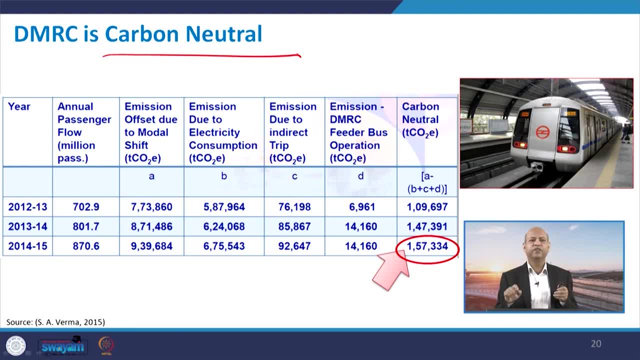 Carbon neutral means there is no addition of carbon emissions because of metro running on the rails, For example. this is the emission offset due to modal shift, So this is more than the emission due to electricity consumption, As I said that some people argue that electricity is also being produced by some fossil fuel. 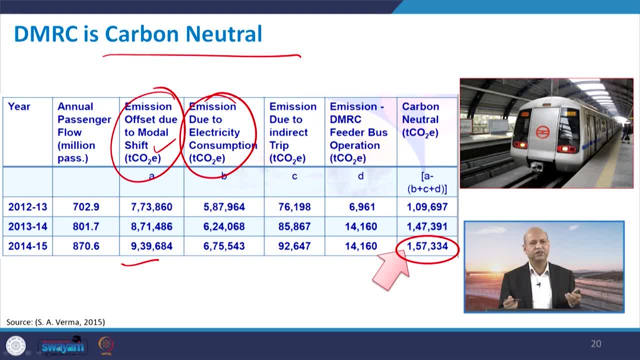 But if you are deriving energy, electric energy by solar panels or maybe from hydro power generated electricity- if you are buying, then you are not adding to emissions of carbon. So that is the thing you can see, that net reduction, Reduction in fatal accidents. 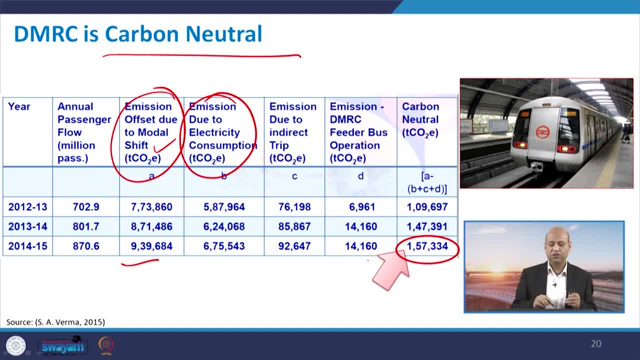 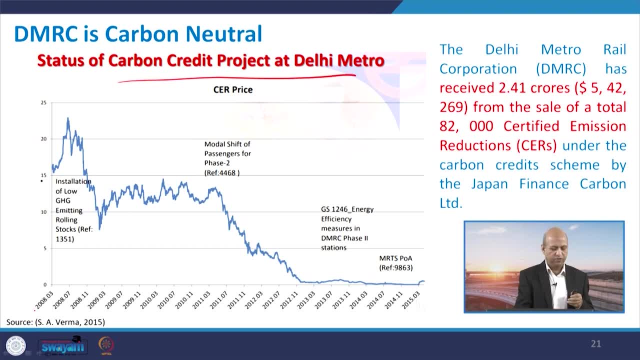 Reduction is there of carbon emissions, So it is not adding to the carbon emissions. In the same sense, carbon credit project have been implemented from very earlier years of 2008 and several crores of rupees saving have been achieved by this particular example. 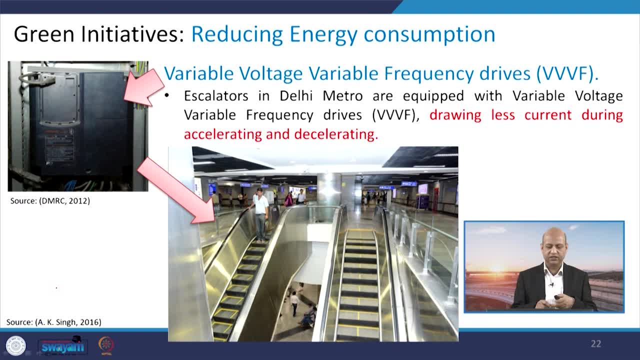 Then there are other initiatives like energy consumption related, these issues in the escalators. So they are having variables- Okay, So variable voltage, frequency drive kind of equipments which uses optimization of energy consumption in these escalators. So that way it is very energy efficient. 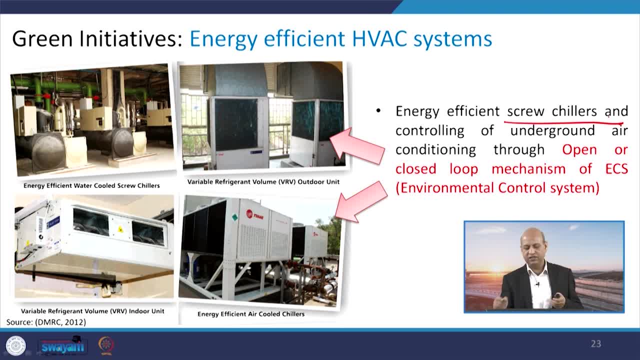 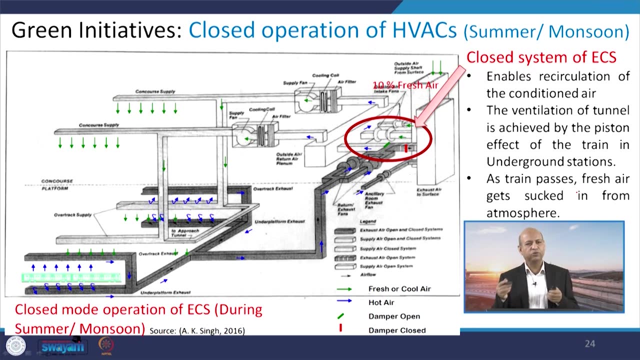 And then if you see these air conditioning and all those systems, so environmental control system is there and they monitor every kind of thing, whether it is moisture level or humidity or thermal, And the controlling system automatically starts some equipment to get the fresh air or it. 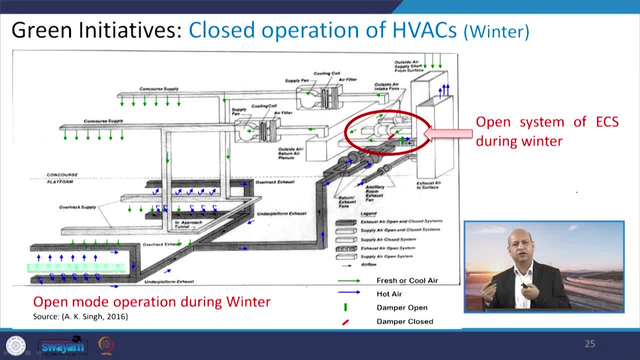 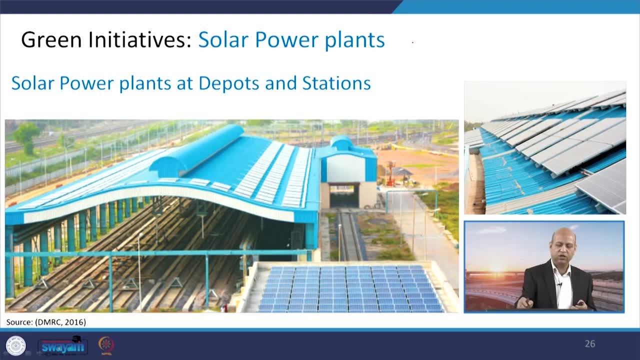 starts to add to the heating processes. if, like in winter, if some, at some pockets, temperature goes down. Well, in solar power plants have been added in this particular, depots and stations, So the roofs have been converted into with solar panels. So a lot of energy is being produced by these initiatives. 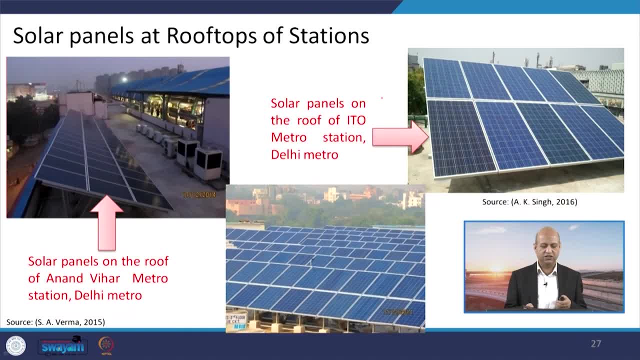 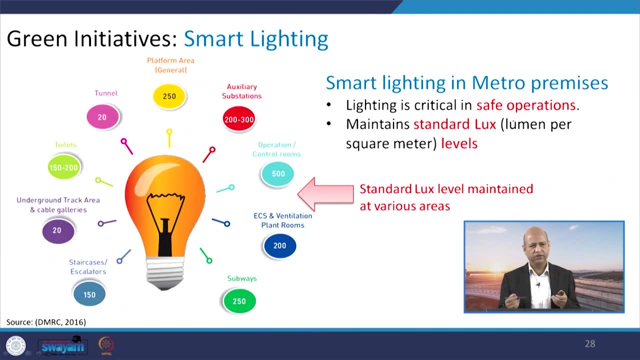 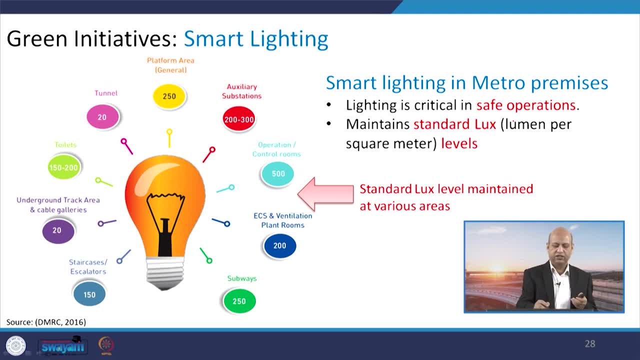 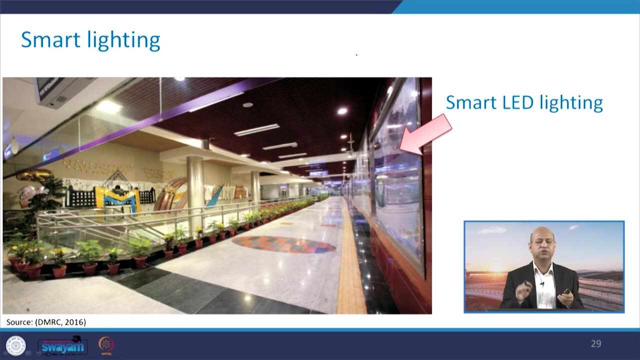 these solar panels to generate the electricity And smart lighting have been implemented. So the saving of energy as well as means where how much illumination is needed. so that way, software have been implemented to have the right quantity of the light, or illumination of the light. 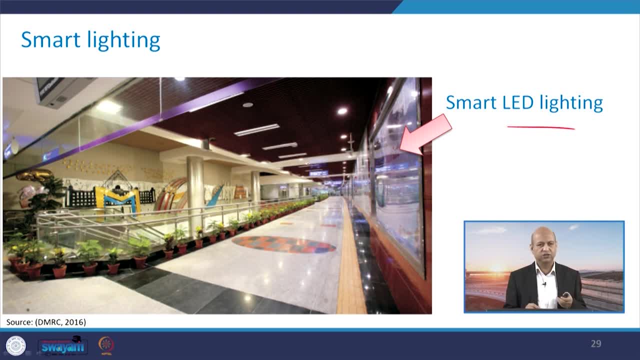 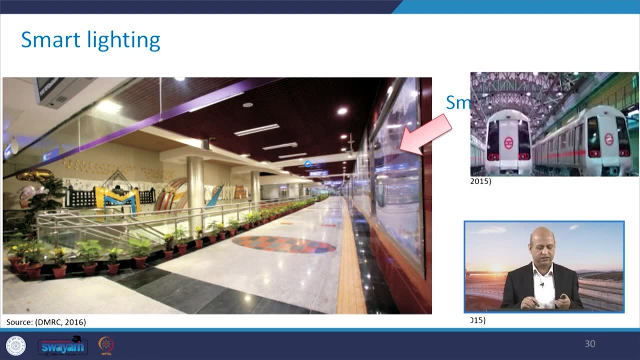 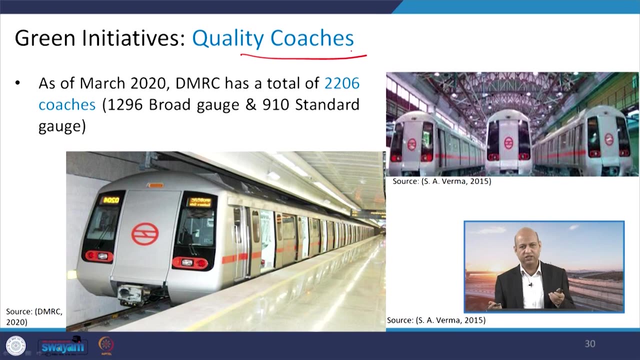 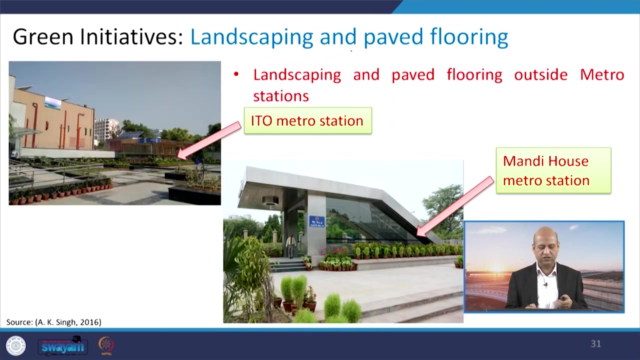 So see these smart LED lights have been used. so very less amount of power consumption, but very good lit. area is there lighting? And then quality coaches, because comfort level should be there for people to travel. so these are the quality coaches which have been used in this DMRC system. 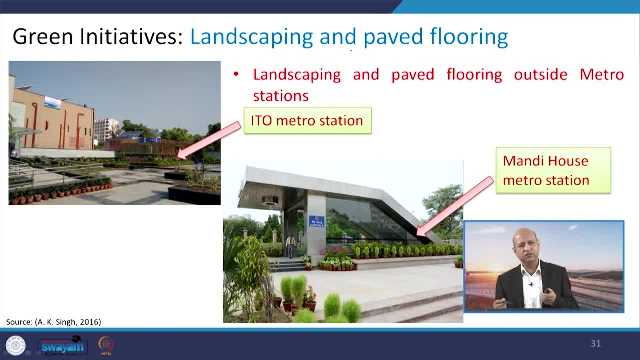 And there are landscaping and paved flooring means the aesthetic value has also been added. There are like water harvesting. all those things have been integrated with each other. so see these look so beautiful- Mundy house metro station. so means people feel very good. 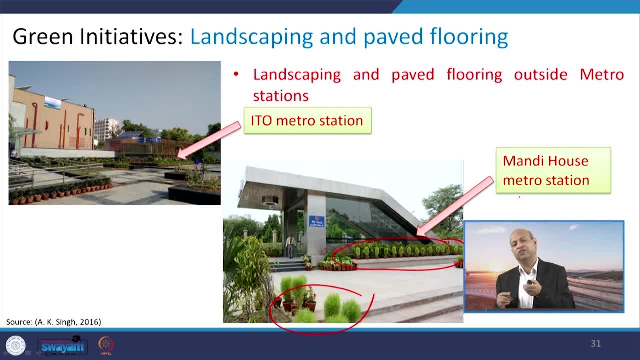 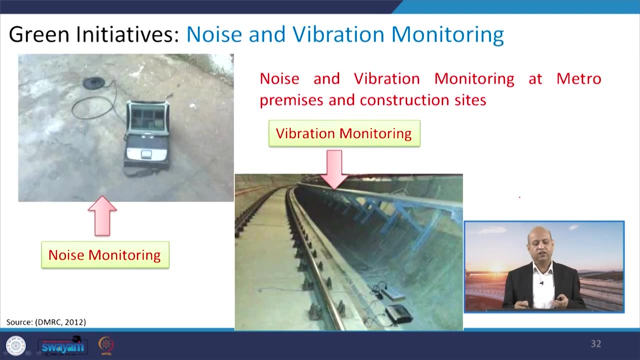 when they approach the station. So otherwise you see, when we go to the bus station It is so crowded and you do not feel good. So those kind of infrastructure facilities really motivate you to go to using this particular system. Then noise and vibration monitoring equipments are also there so that can control the speed. 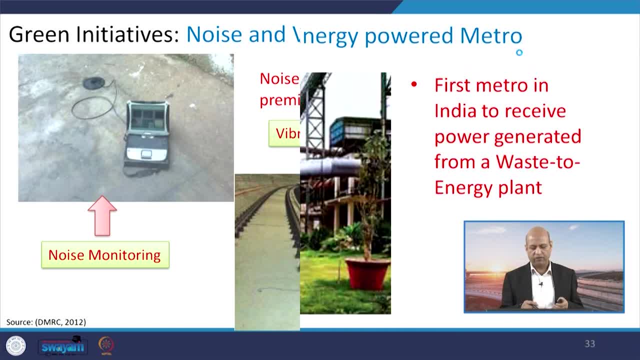 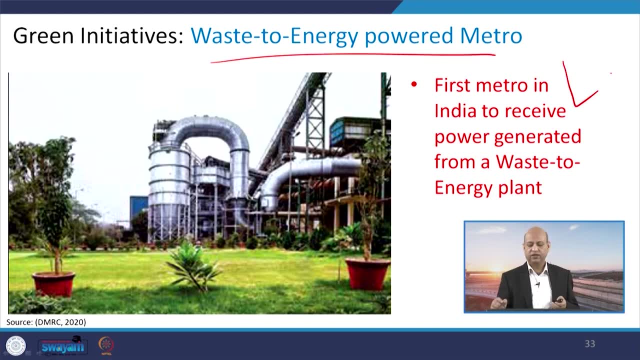 and other issues which affect the noise and vibrations. Of course, this is one wonderful example of waste to energy powered metro. This is the first in India, This particular plant, This particular plant which uses waste material to produce energy as per its calorific value. 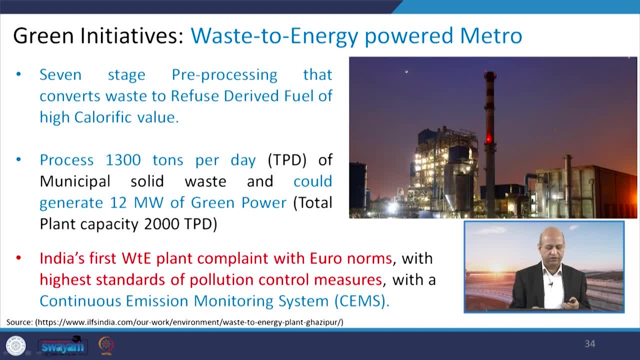 So in this slide it has been given these figures. like 1300 tons per day of municipal solid waste, It is being burnt and converted into energy. plus, there are equipments which control the air pollution exhaust emissions from the stacks, So it is completely clean system. 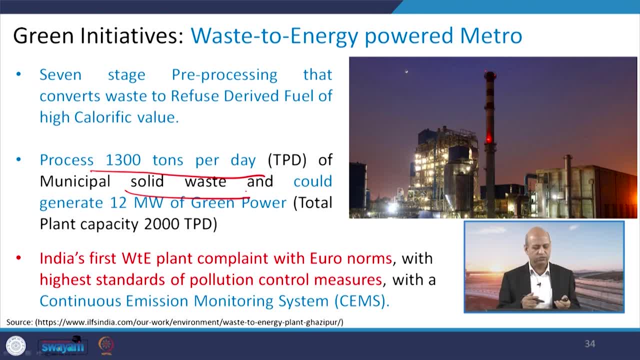 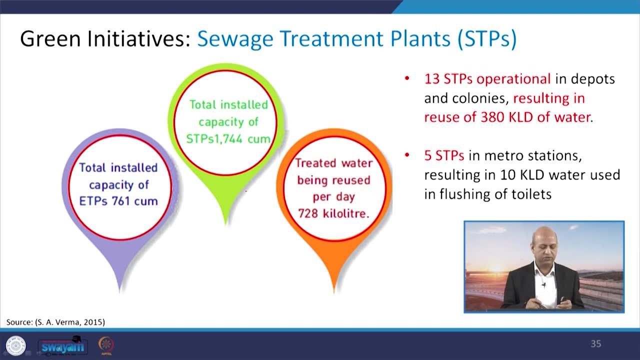 It is not like that it is burning and then emissions are going into the atmosphere. It is not like that. So good controlling of air pollutant system is there and that way this is a green initiative, because it is converting waste into energy. So that way it is a green initiative you can call it. 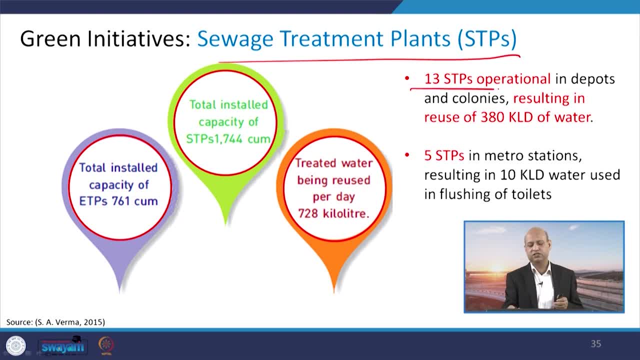 Then sewage treatment plants are there, So 13 STPs, or sewage treatment plants, are there. So, as a result, they are using around 380 kilo litre per day of the water, So that is wonderful achievement. in that way, Affluent treatment plants are also there: around 761 cubic metre of capacity. 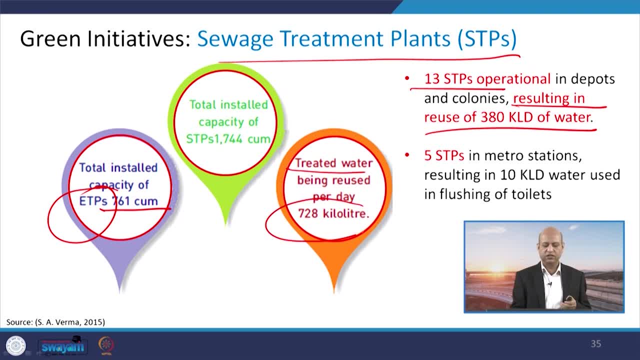 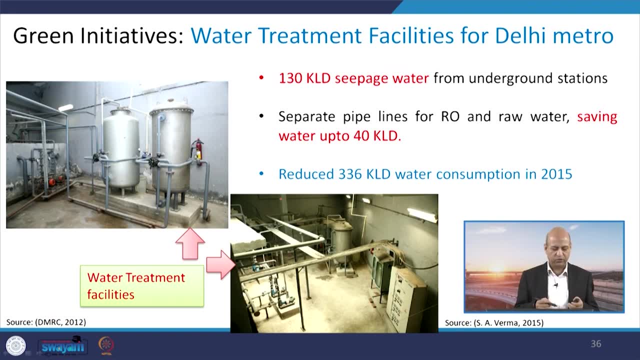 And similarly treated water being reused per day around 728 kilo litres. So those are the things which make it towards environment friendly approach: Water treatment facilities. So in underground there are some seepages, some water losses, so those are collected and they are treated and they are reused in the system. 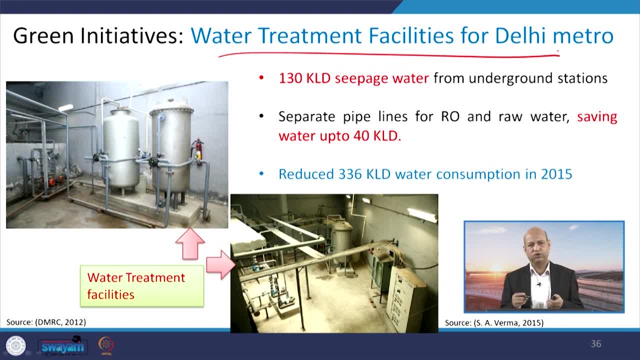 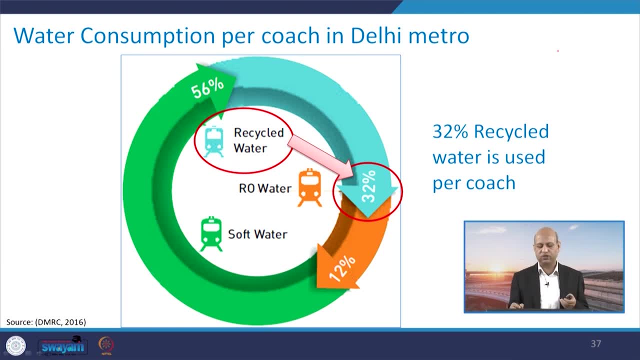 So RO system is there. plus this seepage, water is again made proper to circulate, So that this picture shows how much water is being recycled. 32 percent of the recycled water is being used. It is a big quantity, in fact. 32 percent is not less. and this much only RO water is being 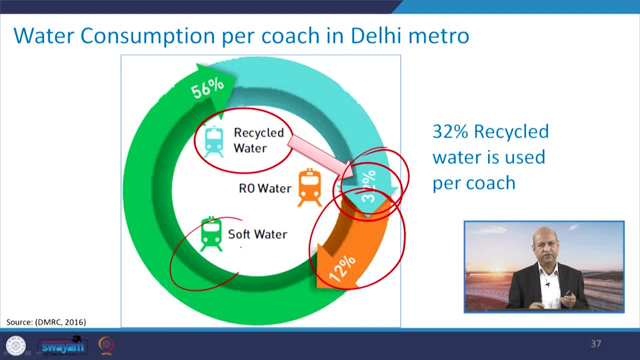 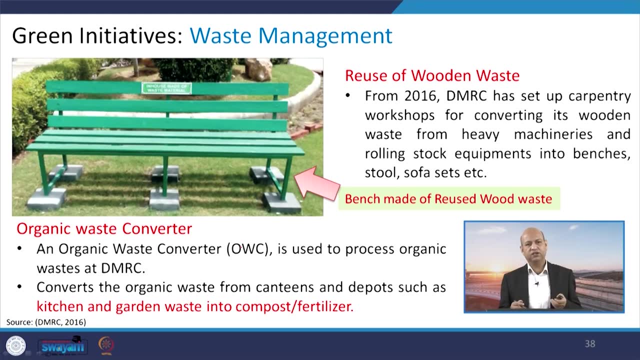 used and the 56 percent is the soft water. So that way optimization in water usage has been achieved. Waste management- Another example- is like. there are lot of wood or other things which are sometimes wasted or outdated. So the DMRC has set up a carpentry workshop to use that discarded wooden furniture. 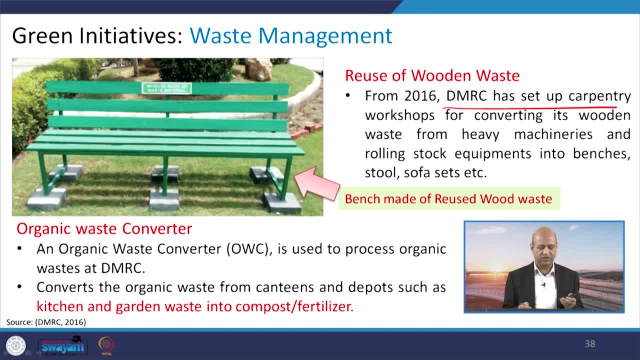 And they again try to make some useful things, for example some bench by this reused wood waste. And then organic waste converter is also there That can process the organic waste of the DMRC And it can be taken from the canteen or depots and then maybe manure etc and for kitchen. 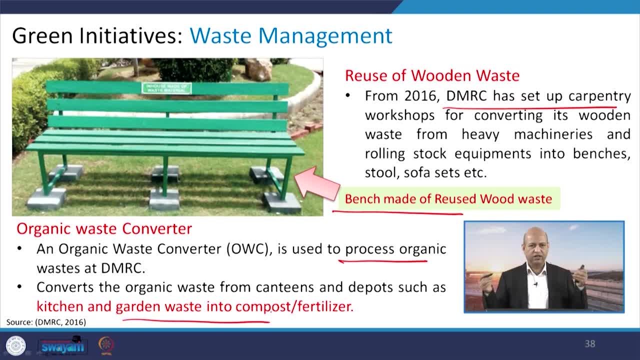 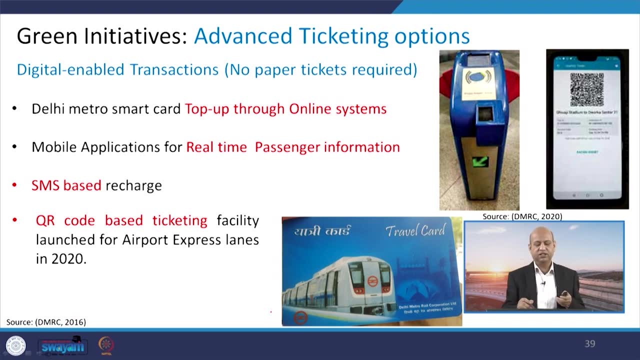 garden. those kind of waste material has been converted into compost or fertilizer So it is again used for gardening purposes. So that way you can see the recycling of lot of things are going on in DMRC. That is big achievement. Also, ticketing options. 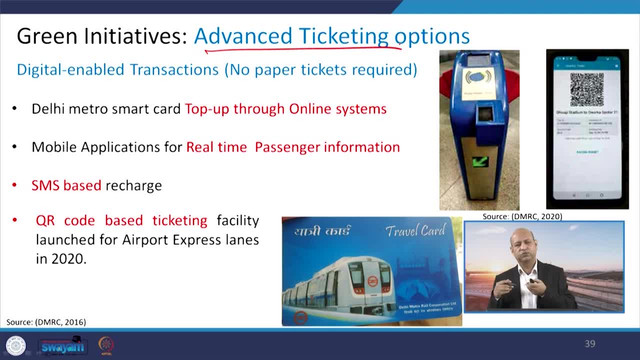 So there are options of advanced nature, like you can use your mobile or these cards, etc. So there is no use of paper tickets and that way you are saving the trees. So that is again environment friendly approach and SMS or QR code kind of technological applications. 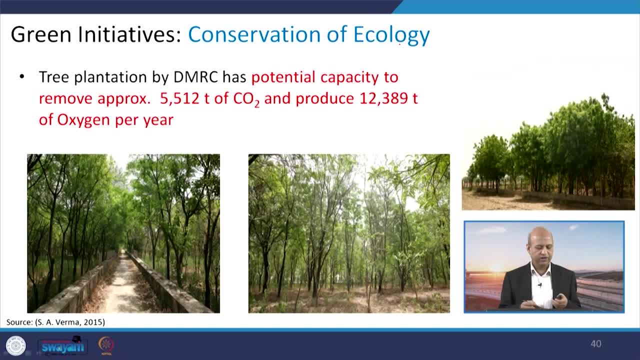 have been integrated with ticketing and traveling from one place to another. Then DMRC has also invested a lot for conservation. So this is a big achievement, Thank you. So let us talk about the CO2 emission. So the CO2 emission is the emission of carbon dioxide from a tree or a plant. 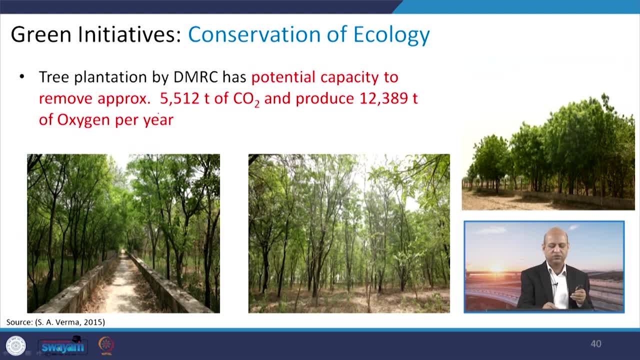 So it is a big issue. It is a big issue. It is a big issue because the CO2 emission is the emission of carbon dioxide from a tree, So it has a lot of benefits. So the CO2 emission has been used for conservation of ecology. 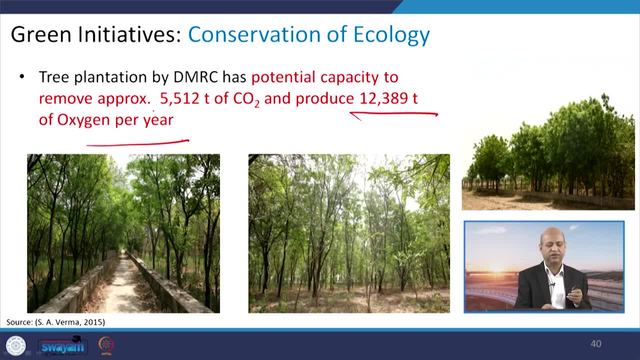 So it has planted lot of trees and they produce around 12,000 ton of the oxygen per year and they remove around 5,000 ton of the CO2 means, because it is a sink. CO2 is used by plants, as you know, for producing their own food and they also give oxygen. 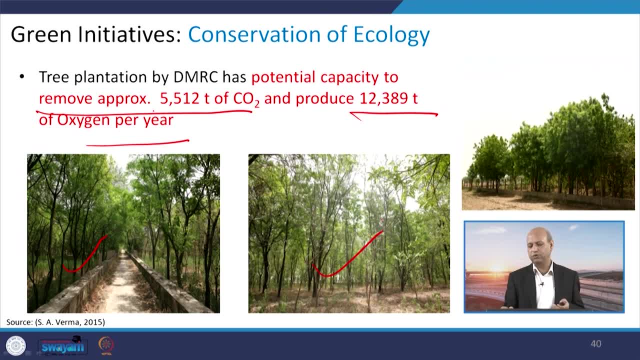 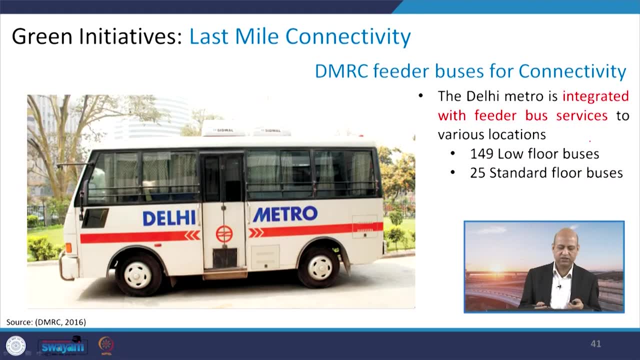 So that way, lot of plantation activities has been funded by DMRC, so that that is again wonderful initiative, Thank you. in terms of the environmental protection, Last minute connectivity or last mile connectivity related facilities or infrastructure have also been taken care of by Delhi Metro. 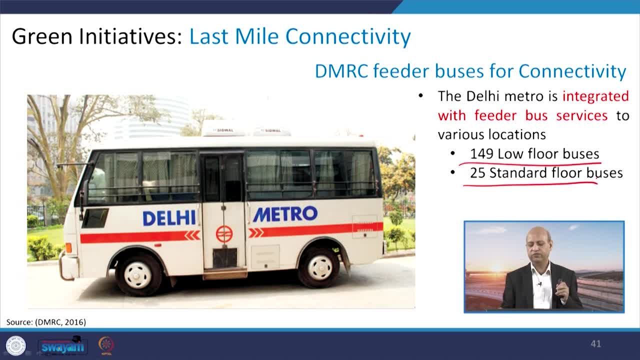 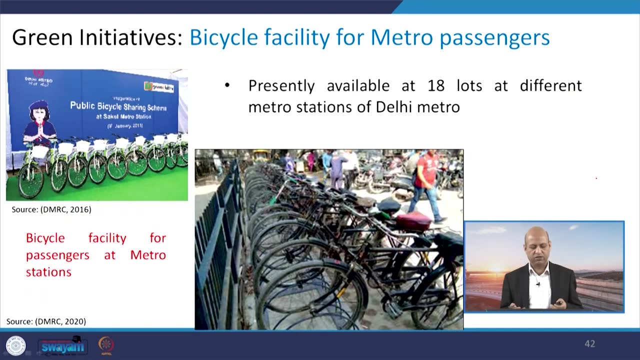 So around 149 low floor buses and 25 standard floor buses have been used for this last mile connectivity, so that people do not feel or to wait for some other automobile to go from metro station to their destination. Then there are initiatives like bicycle facility at certain locations, around 18, lots of bicycle. 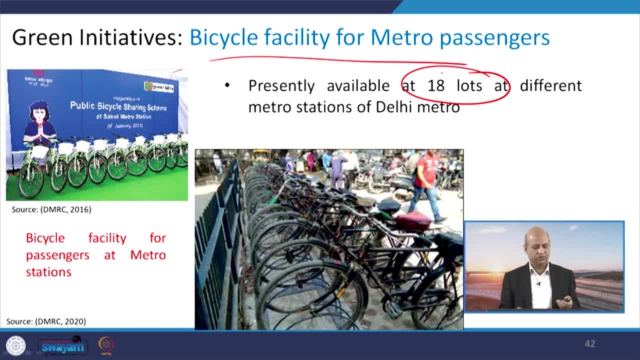 facility are there, You can just hire the bicycle and you can drop it at another station. So that way means it is like that. It is like benefit to the health as well as there is no emissions. So this non-motorized vehicle categories have been integrated with Delhi Metro system. 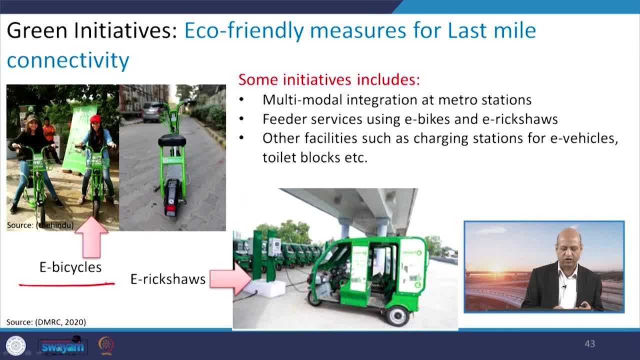 So that is wonderful example. Similarly, e-bicycles are also there, e-rixas are also there, So all those multi-modal integration have been achieved in metro stations to facilitate the passengers. So e-rixas are there. and then charging stations are also there, so that they do not need to. 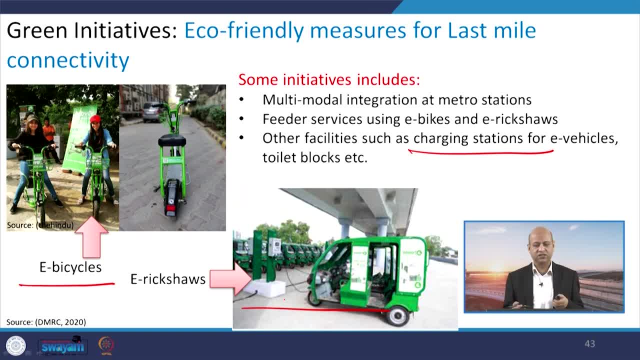 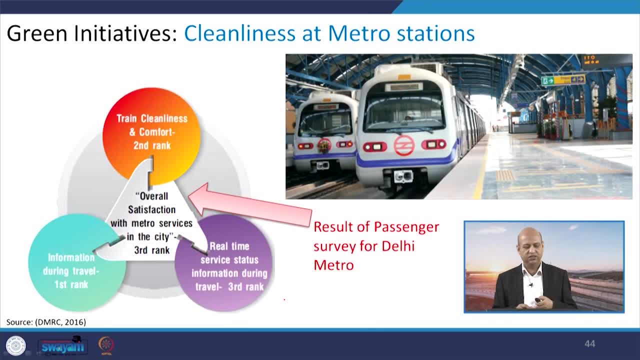 go here and there And they get opportunity to charge their e-rixas batteries very conveniently. Well, then again, if you see the cleanliness and comfort level. so there was a survey and on the basis of that survey, it was known that information during travel, that is the very 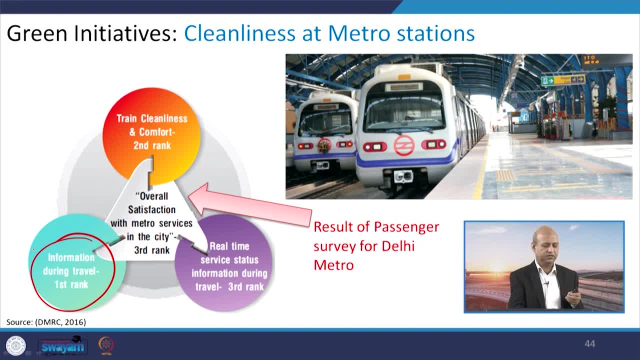 good means first rank. people say that this is the best category or best practice, for best aspect of this Delhi Metro system. Then cleanliness, of course all these are of high rate, but if you rank in relative so, cleanliness is the second and the real-time service is around at the third rank. but they 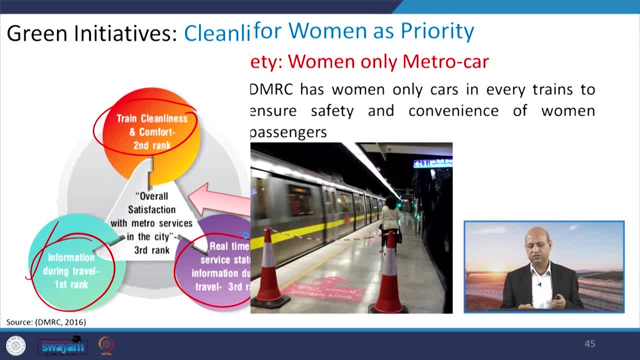 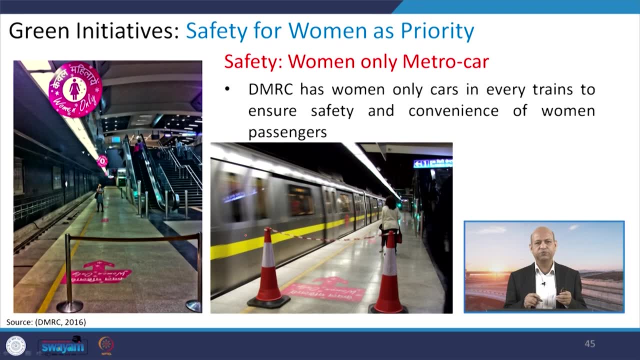 are of very good quality. only the comparison of these three variables are there. Plus there are certain coaches or cars which are dedicated to women passengers. so for convenience, for their safety, there are dedicated cars only for women. so this kind of facilities. 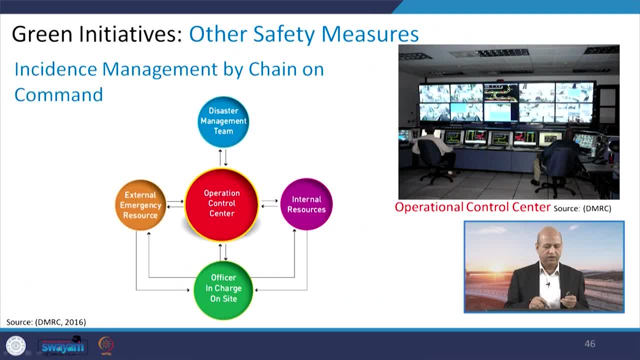 also in each metro there, If you see the safety measures. so again, control system is there and they constantly monitor. automatic systems are there of any kind of deviation from protocol. so all kind of possibilities are there. There will not be any kind of fatal accidents. 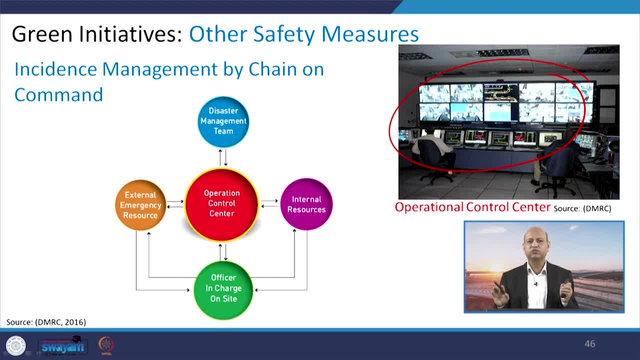 So it is a very good thing, Thank you, Okay, Very. 2. meanwhile, if there are any accidents, the metro will stop automatically. you might have read sometimes in newspapers that there was power breakdown because of some unknown reason and then metro got stopped and there was but some backup power. so that comfort. 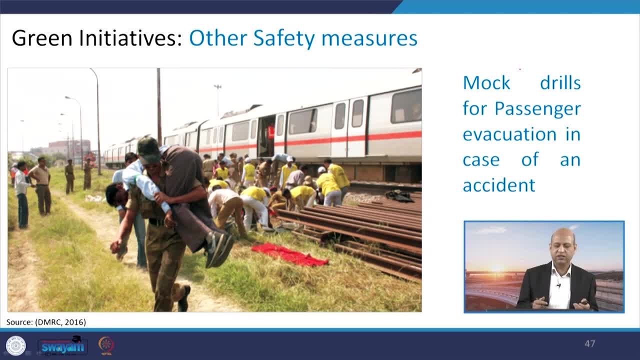 level was not reduced for the passengers. Plus, there are some mock drills if something happens, because accidents are accidents, they do not come with the warning. So if somehow, if a traffic police becomes, your safety of your passenger becomesFinally coming, just do not return onading. 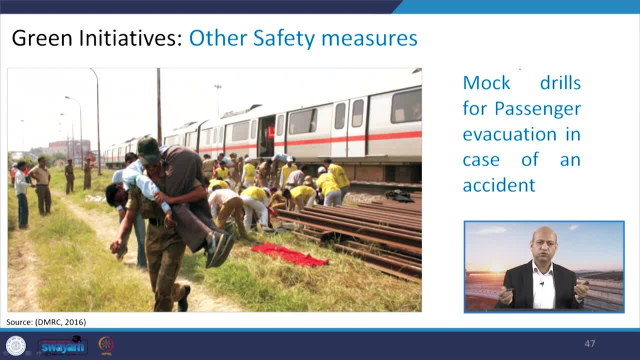 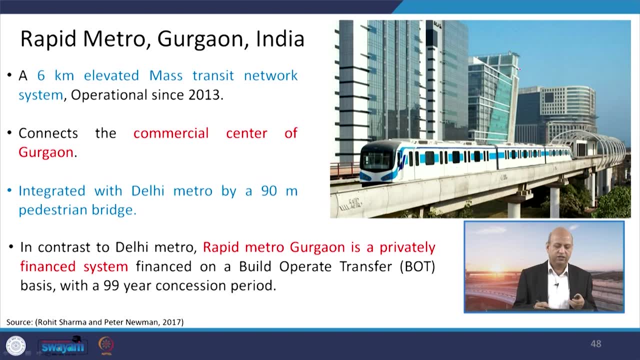 And those kinds of things happen, then how to rescue the people. so those kinds of mock drills are also conducted by DMRC time to time. Well then, there is the integration of rapid metro of Gurgaon, as I said, and this is around. 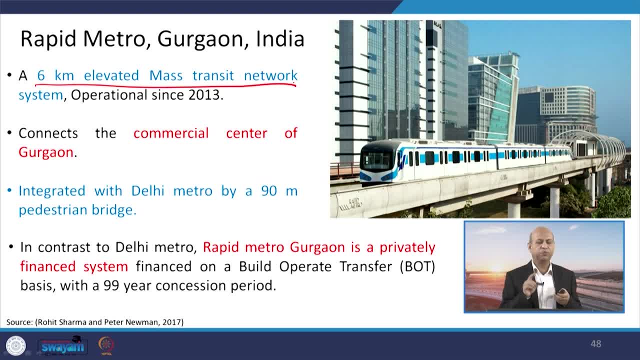 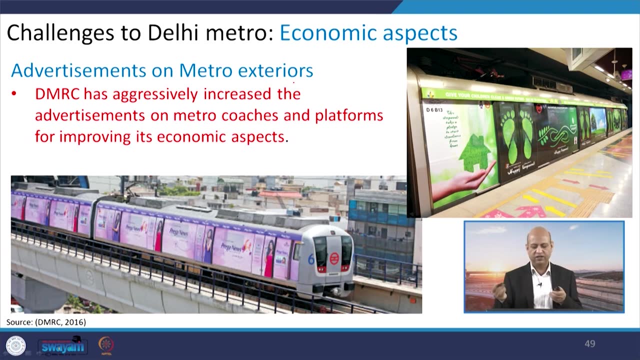 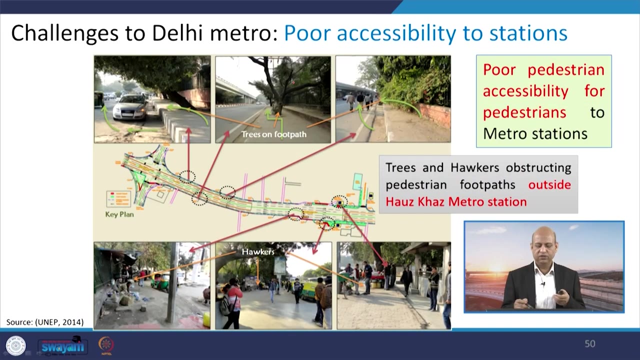 6 kilometer elevated mass transit network and it is operational since 2013.. Wonderful part is that it is managed by privately owned agency and that way, the integration of this Delhi Metro Corporation and that Gurgaon's rapid railway system is there. Then there are certain challenges because poor accessibility related things have been 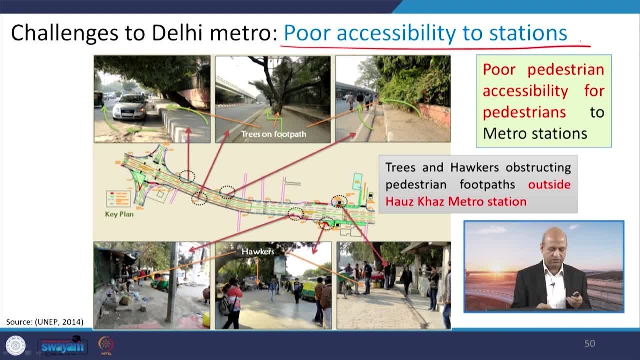 observed and people have complained. So, as a kind of challenge or as a kind of a scope for improvement, I would like to share with you- like at certain places you can find that like there are hawkers and people who mobility is not so good. 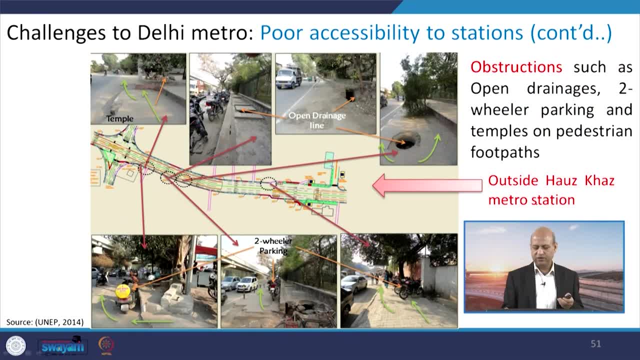 In that sense you can even see these like outside the hoskos. some pictures have been taken, open drainage and the potholes, and then there is a huge gap between this platform, walking pedestrian and the level. So those things are there and they should be taken care of. 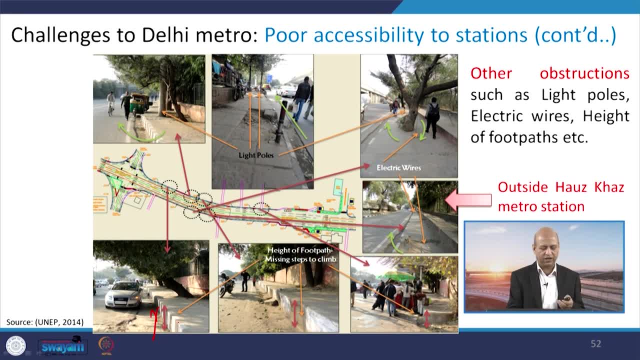 See the height. without one more step, it is very difficult to climb this kind of you know footpath. So, and then there are you know trees in between. So again, if somebody- nowadays people have a habit of you know reading something text- 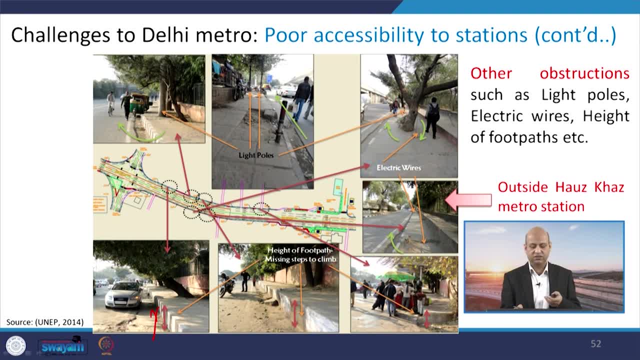 message, etc. there may be a chance of hitting this tree. So when Metro is planting so many trees, maybe they can take permission from the forest department to remove or to transfer this tree from one place to another so that the safety aspects are met for them. 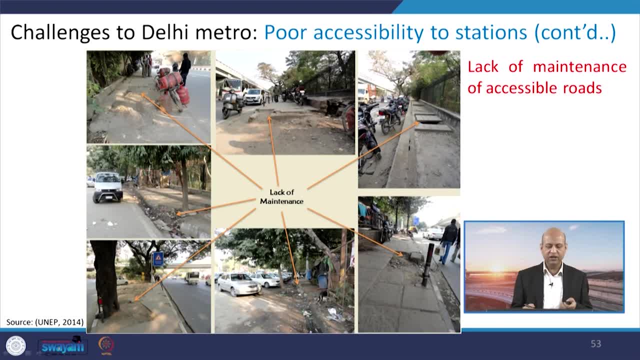 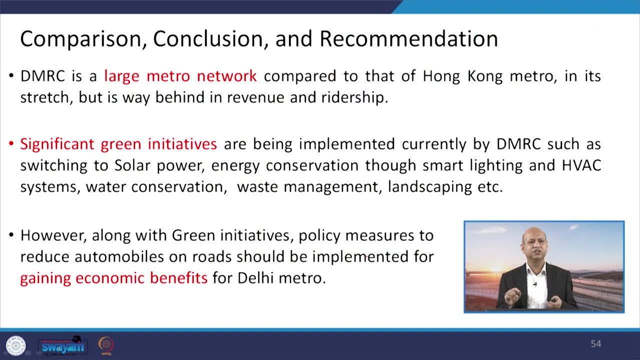 Okay For the passengers and people. Similarly, other you know pictorial representation are given like these kind of. these are the not good footpaths and these broken tiles or maintenance is not good on accessible roads. So those are the challenges where scope is there for the good improvement and I hope 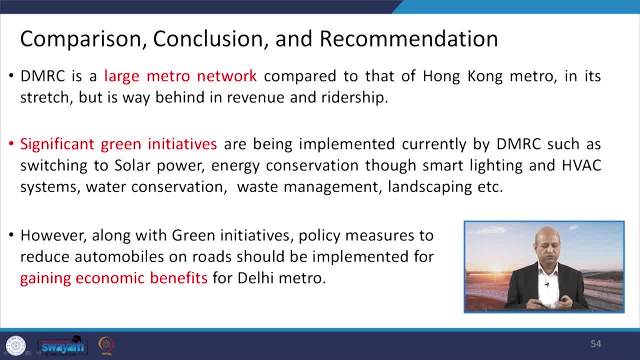 in near future these things will be addressed properly. So if we compare our DMRC with the- you know Hong Kong Metro, Then you know. I mean there is a lot of scope to improve in terms of ridership or revenue generation. 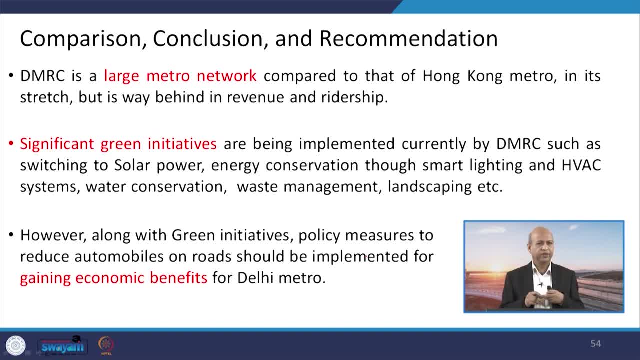 We are far behind from Hong Kong Metro, But significant green initiatives really bring this DMRC at the forefront as a very good example of environment friendly or sustainability aspects, integration into the whole system. Okay, And if we want to recommend something, then we can say that some economic benefits can. 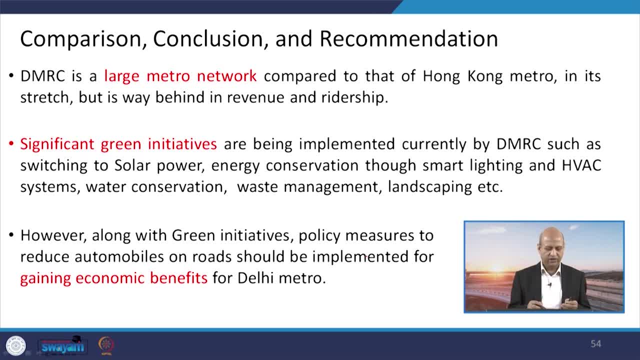 be taken into account and those should be transferred to improve the system. plus more automobiles and those policies should be that the usage of automobiles should be reduced. in that way, those policies should be implemented and those amenities which are not at par with the expectation of the people. 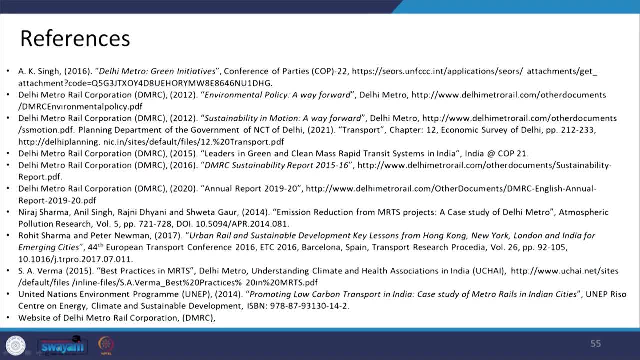 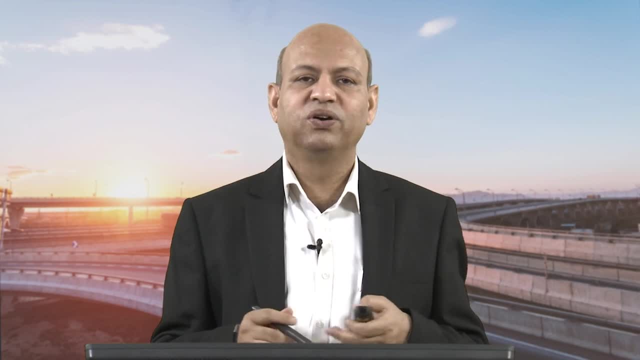 Okay, So that is all for today And this is the list of references. So anyone of you if you want to know more about certain aspect, you can go to references and visit those reference to gain more knowledge, and thank you for your kind attention.